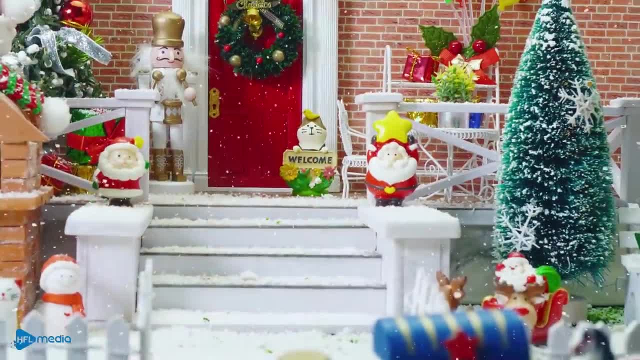 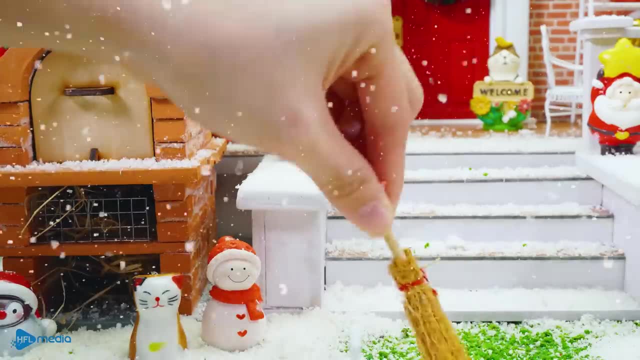 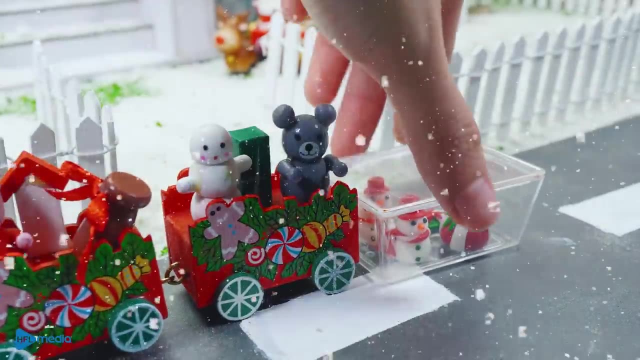 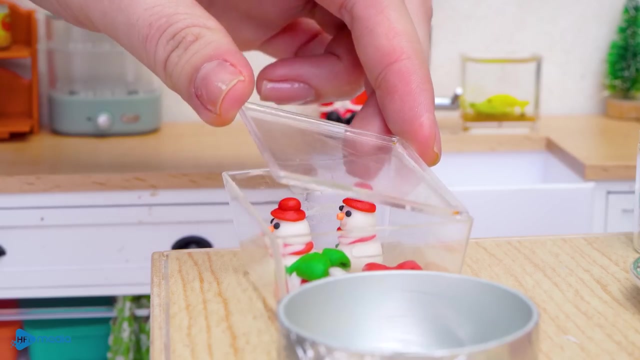 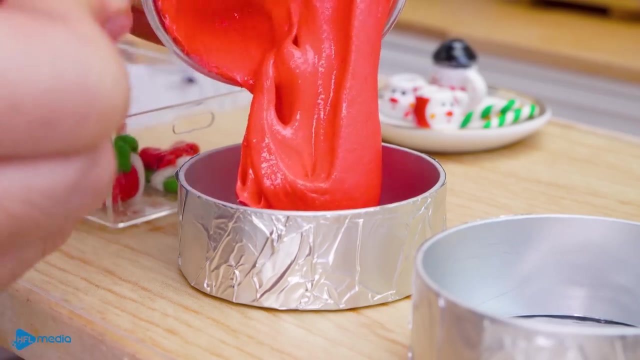 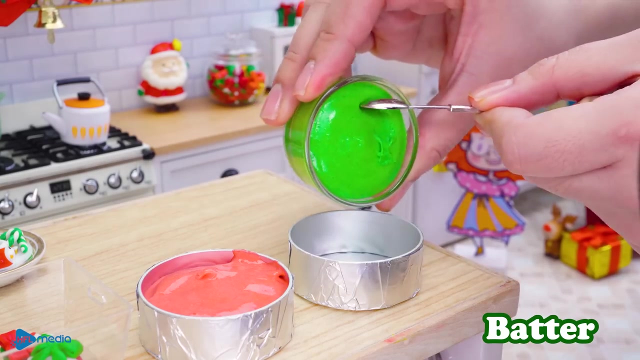 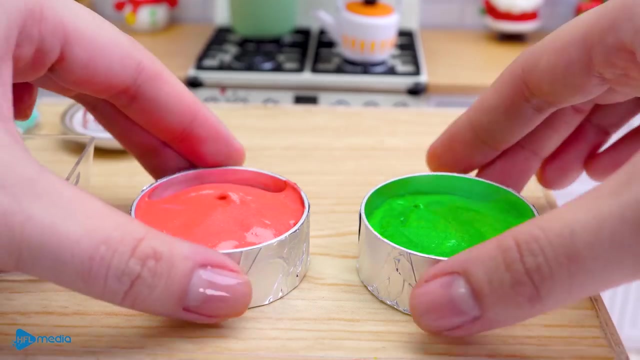 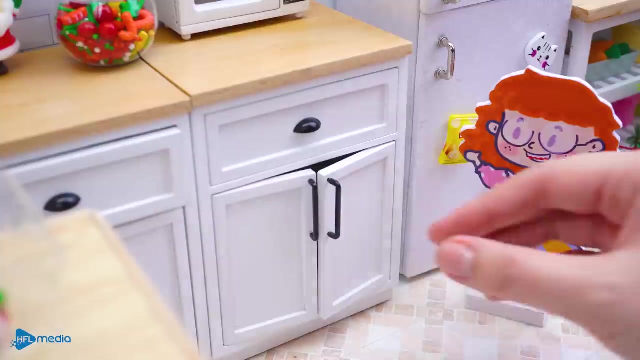 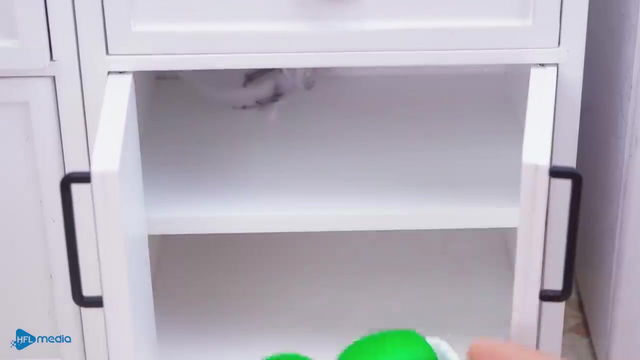 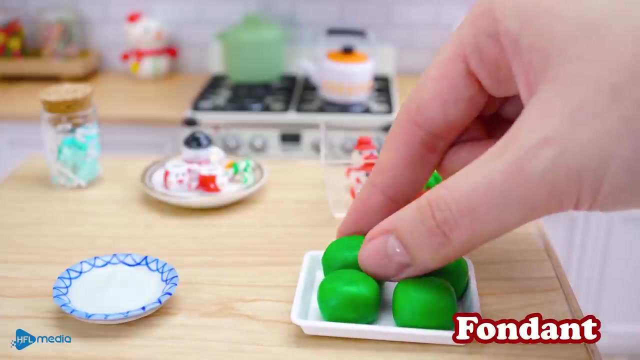 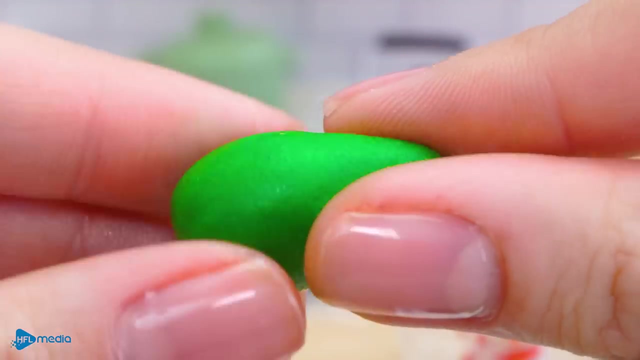 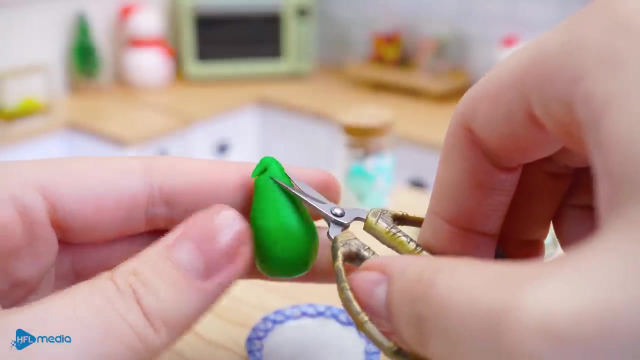 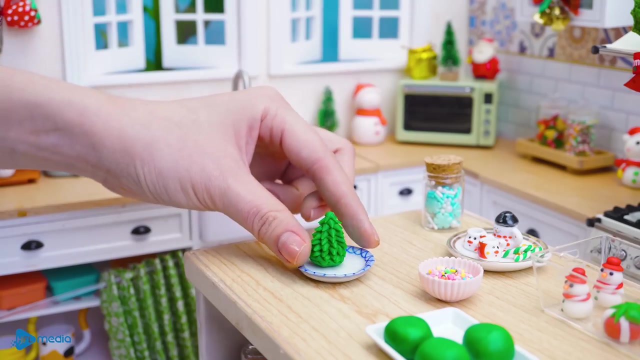 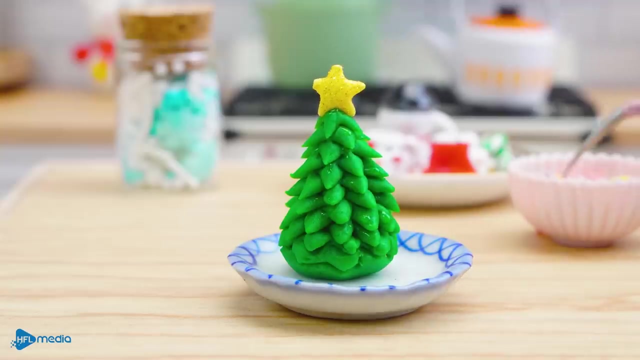 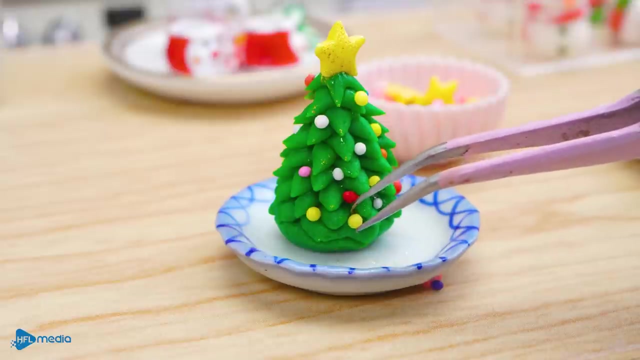 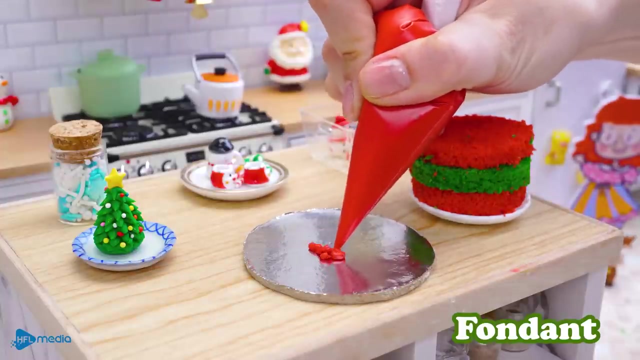 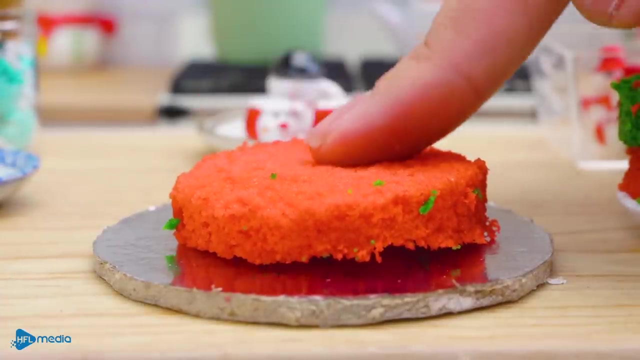 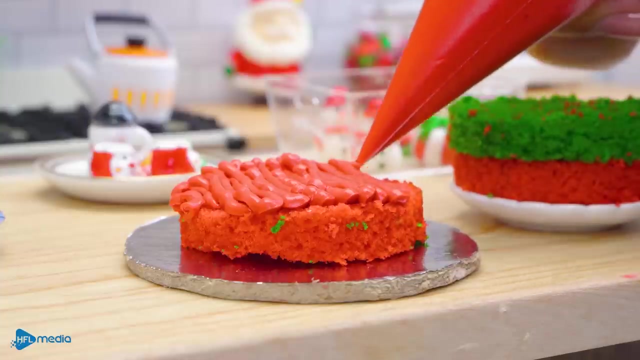 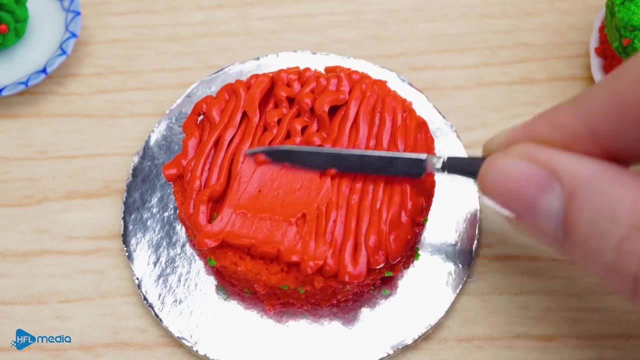 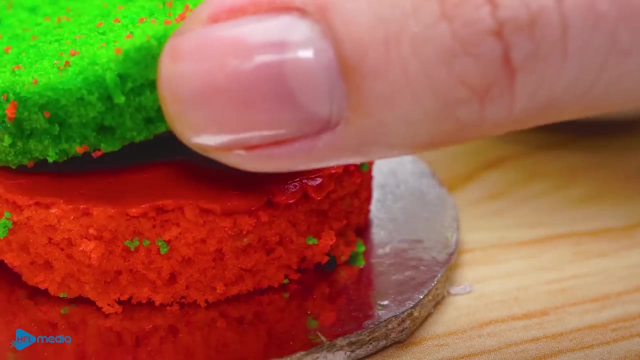 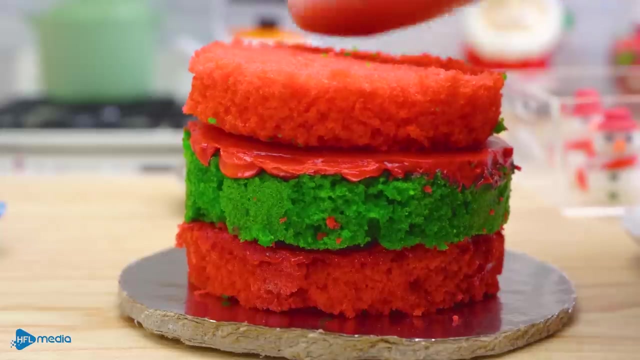 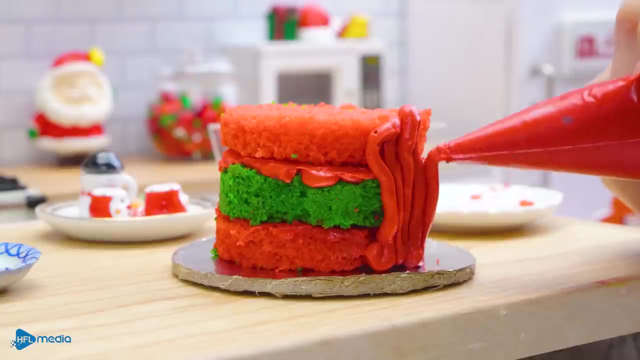 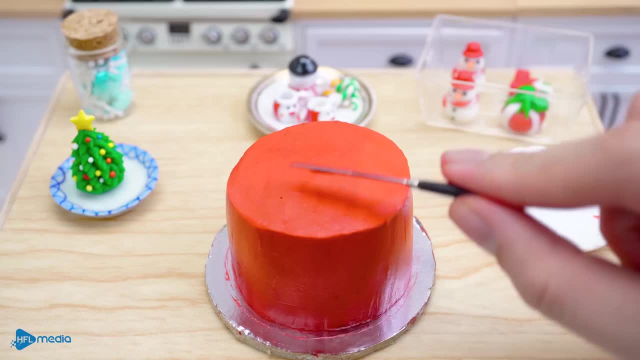 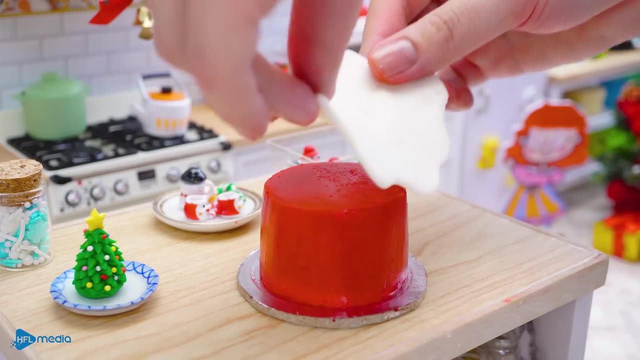 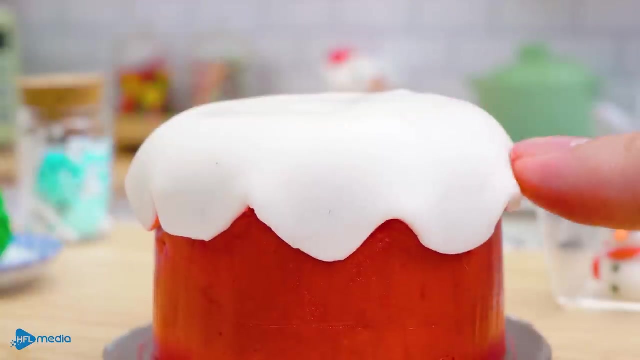 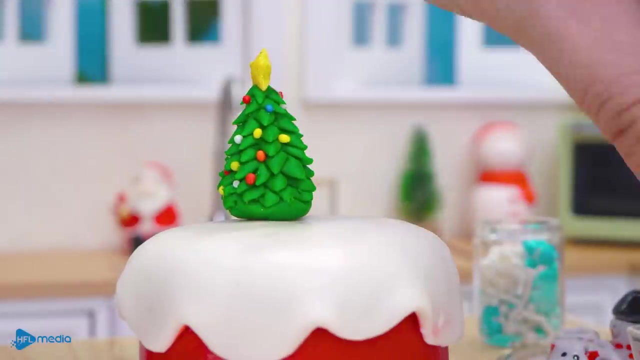 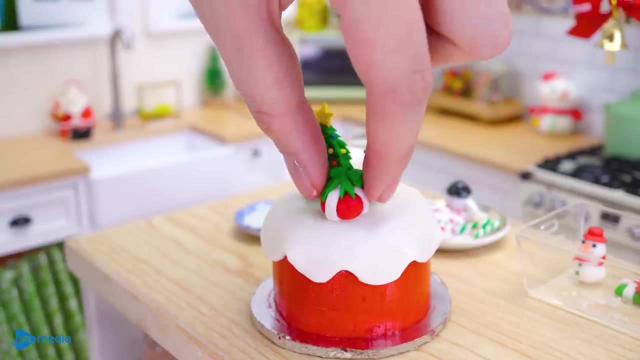 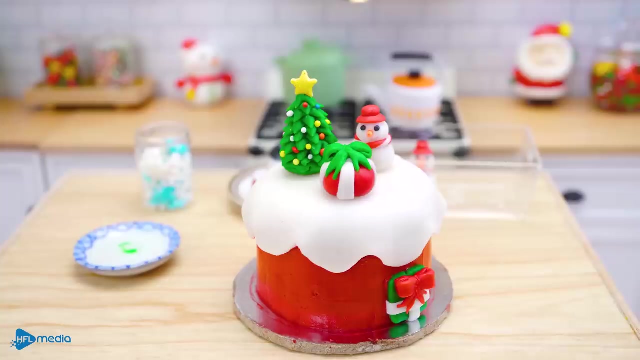 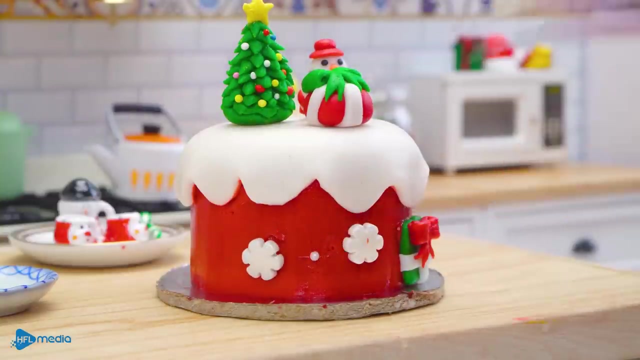 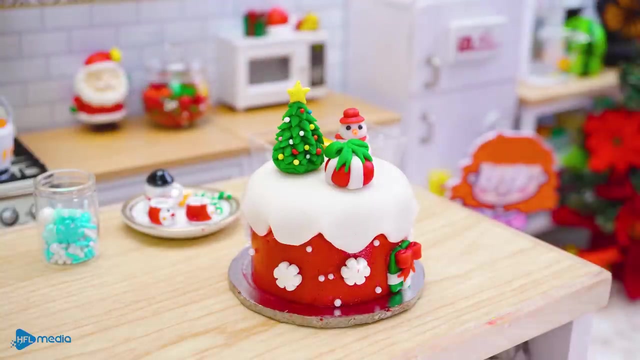 cake with this. so I'm going to make a cake with this and I'm going to make a cake with this. so I'm going to make a cake with this and I'm going to make a cake with this, so I'm going to make a. 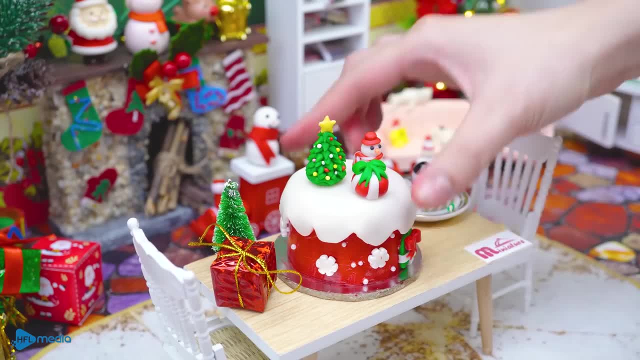 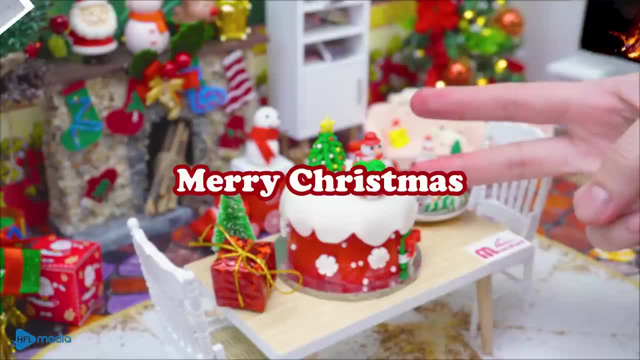 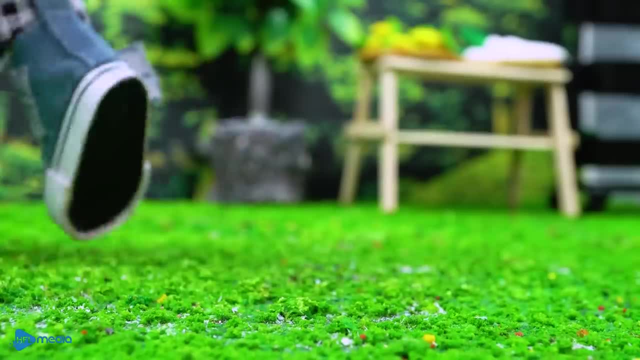 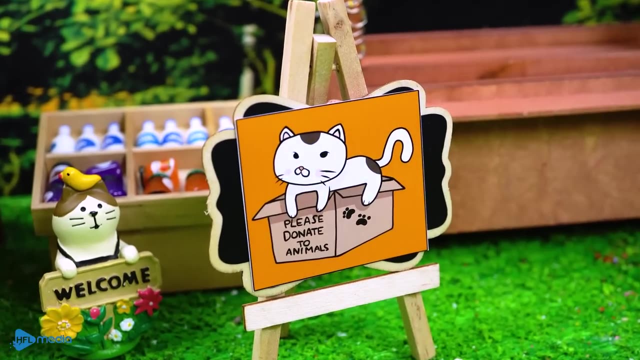 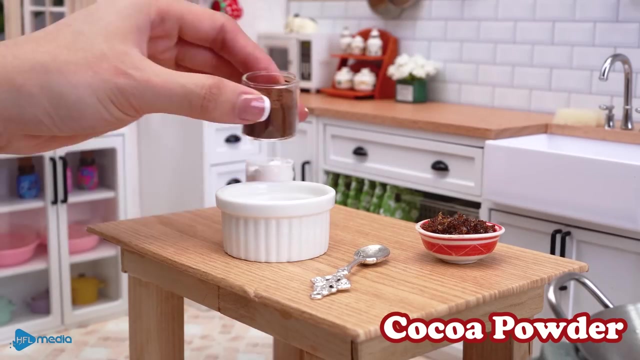 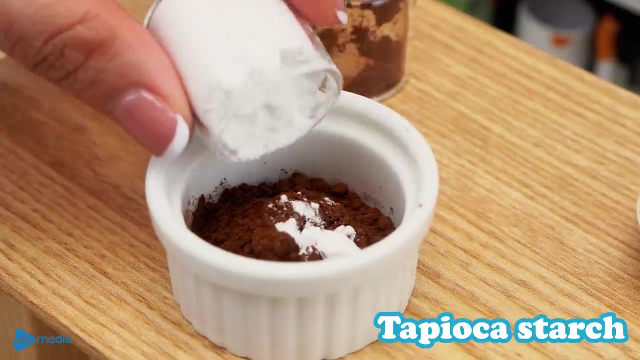 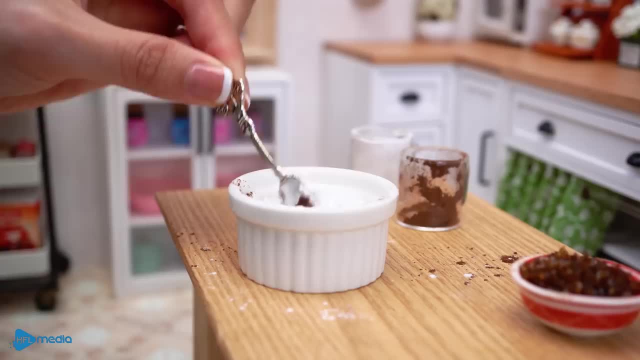 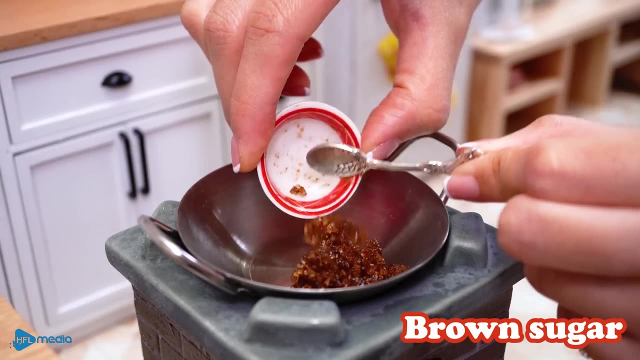 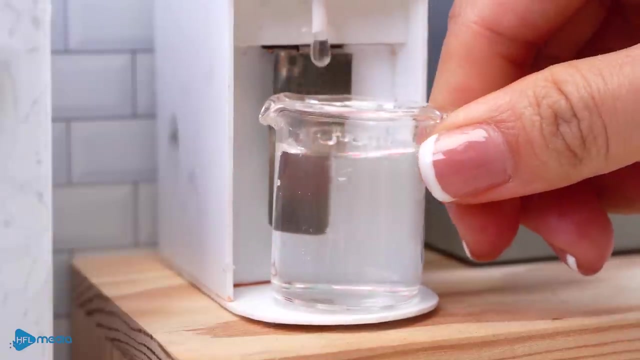 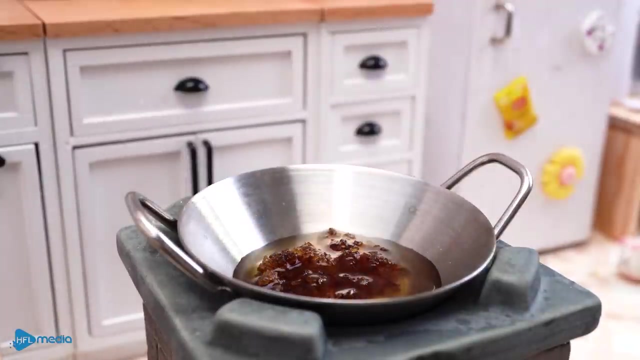 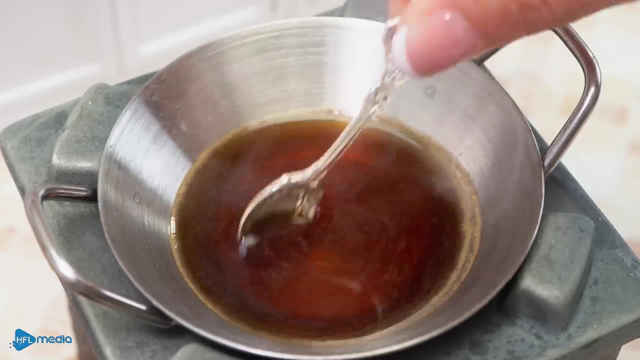 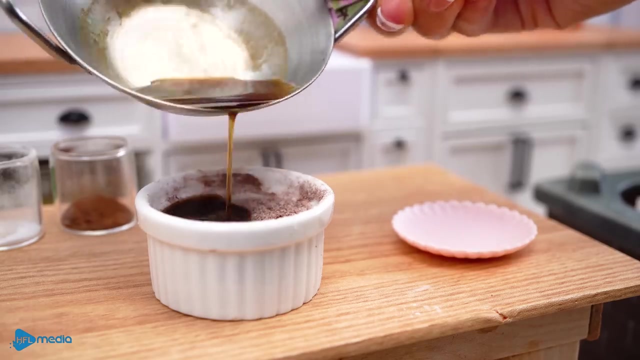 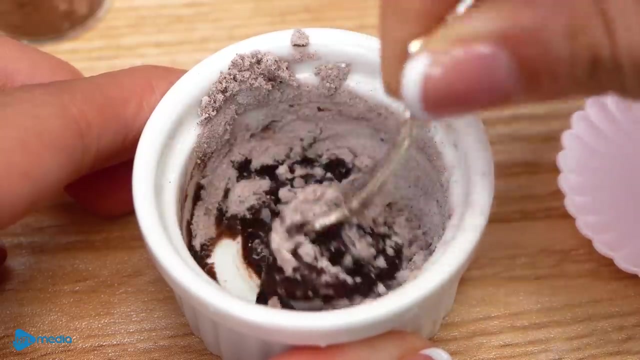 Add ground chicken to the chicken, Add 1 tablespoon of soy sauce and 1 tablespoon of cooking wine to the pan and stir-fry. Add 1 tablespoon of water and stir-fry After 50 minutes. When it's done, pandan leaves. 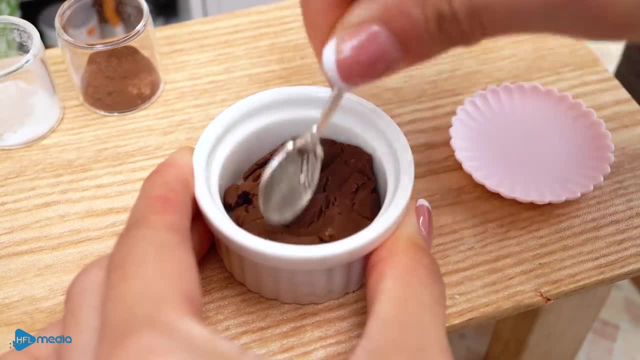 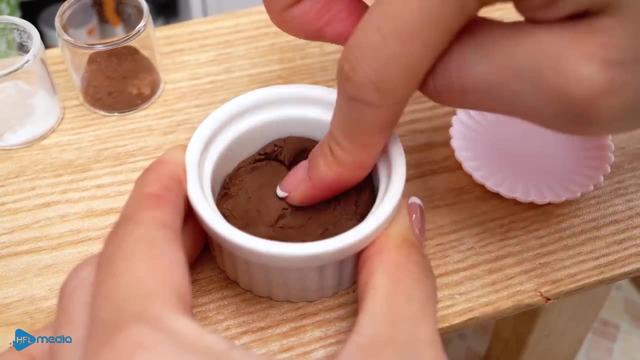 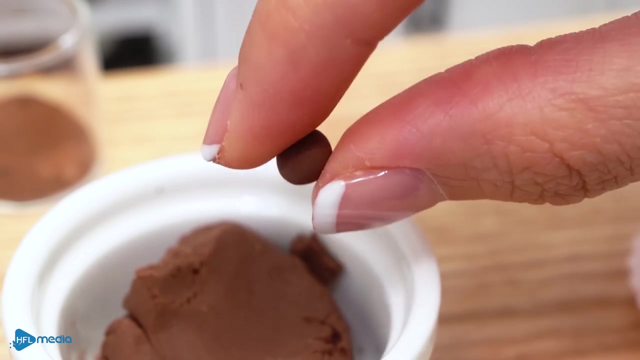 and it doesn't stick to the plate. turn off the heat and let it cool. Strain the gas through a sieve. Sealed Instagram is up to you. See for yourself: ihrehh. 1 tablespoon of sugar. 1 tablespoon of honey. 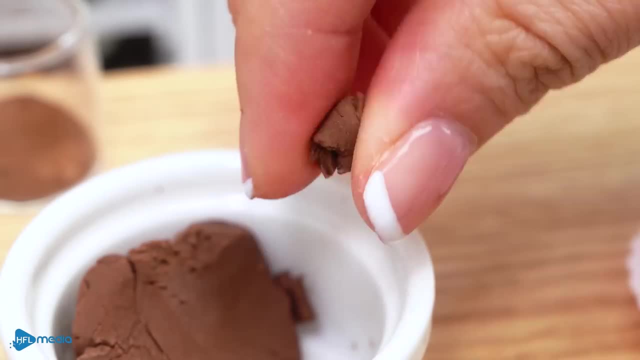 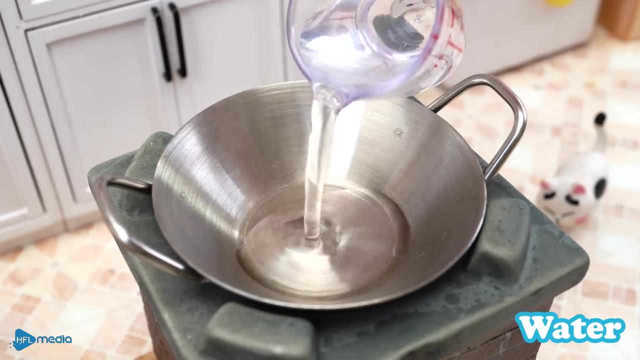 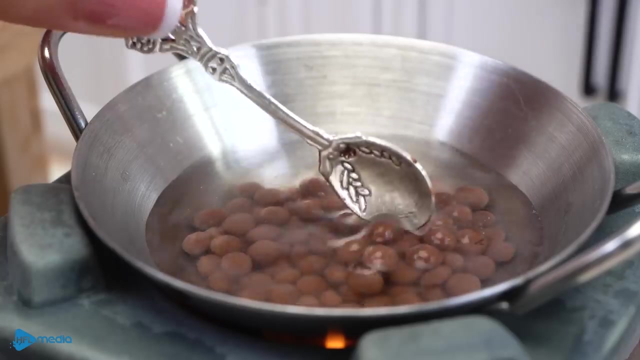 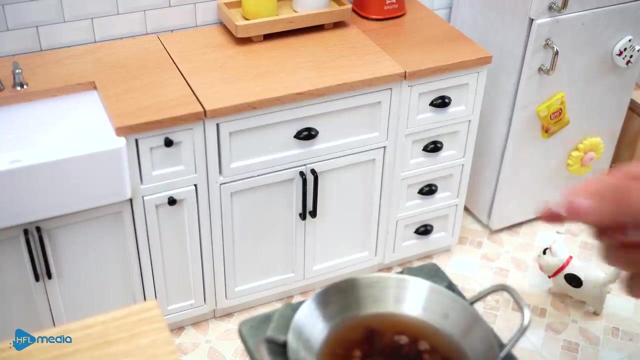 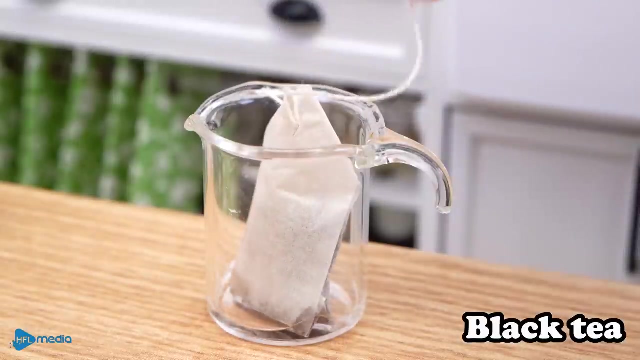 1 tablespoon of vegetable oil, 1 tablespoon of olive oil. 1 cup of water. When the soup starts to boil, turn down the heat. Add 1 tablespoon of sugar. welcome to my channel. Add 40ml of water. 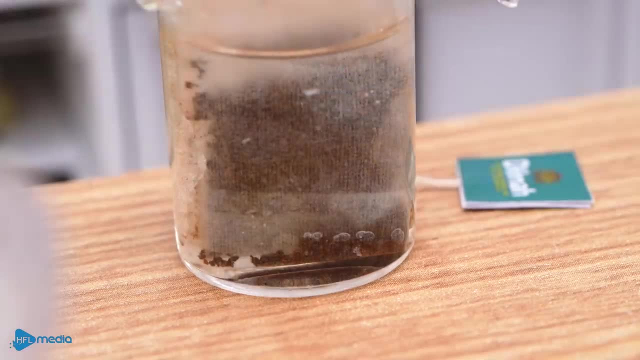 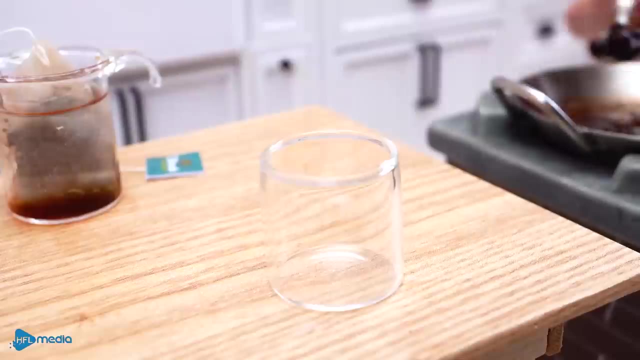 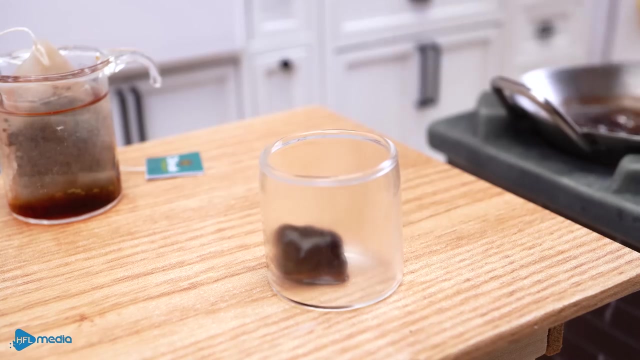 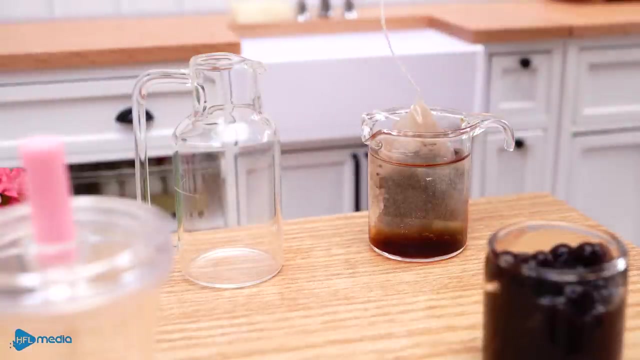 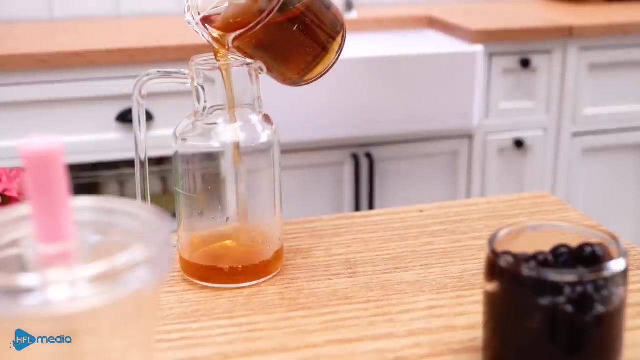 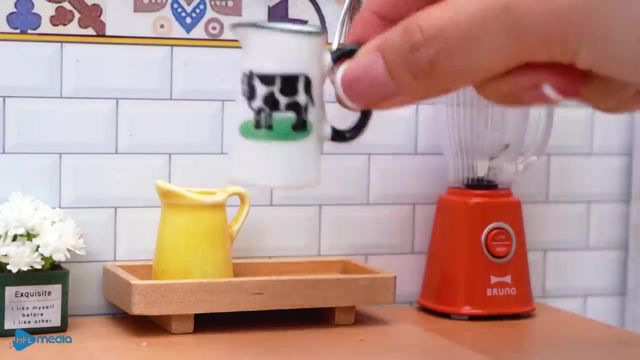 Boil for 3 minutes. Mix the sauce, Add some cooking oil, Add 2 tablespoons of soy sauce. Add 2 tablespoons of oyster sauce. Add 1 tablespoon of minced garlic. Add 2 tablespoons of soy sauce. Add 1 tablespoon of soy sauce, 1 tablespoon of sugar, 1 tablespoon of cooking wine and 1 tablespoon of cooking wine and mix well. 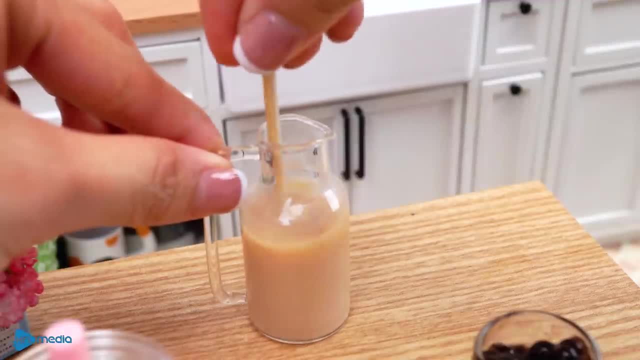 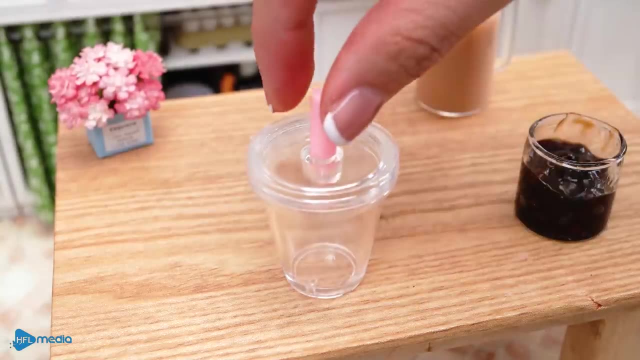 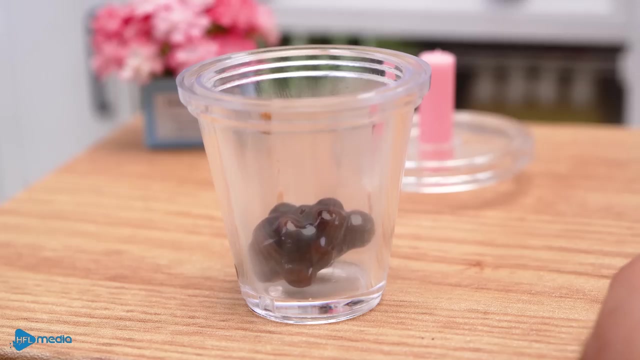 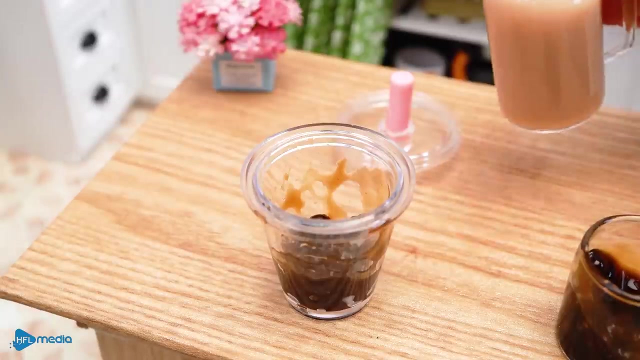 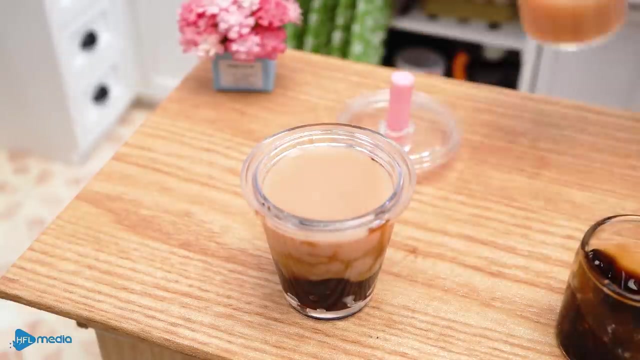 Add 1 tablespoon of soy sauce and 1 tablespoon of cooking wine and mix well. Add 1 tablespoon of water and mix well. Add 1 tablespoon of soy sauce and 1 tablespoon of cooking wine and mix well. Add 1 tablespoon of cooking wine and mix well. 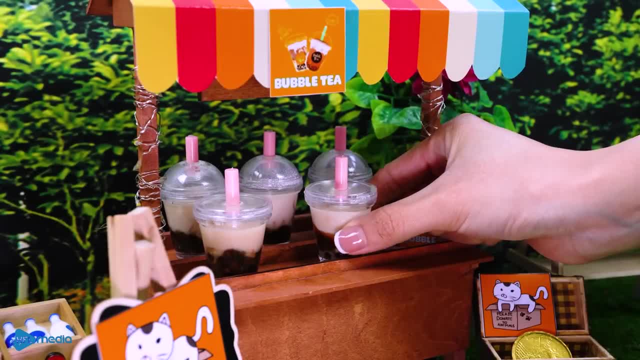 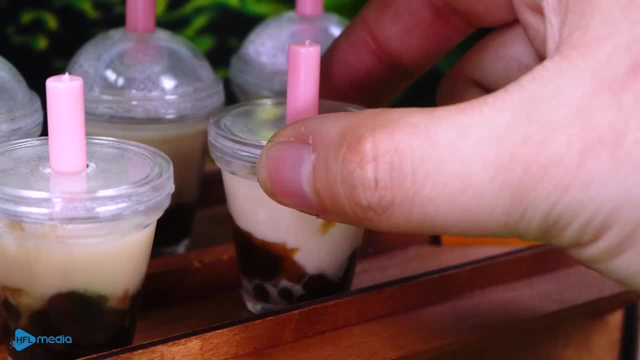 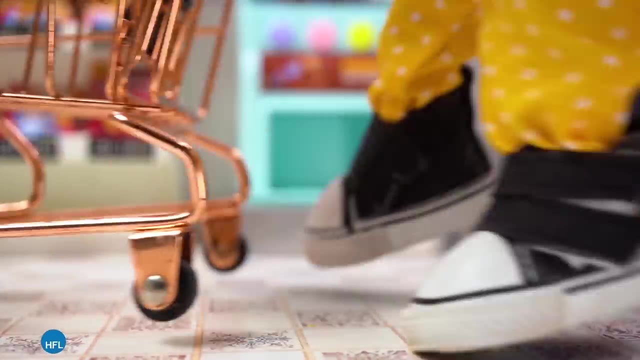 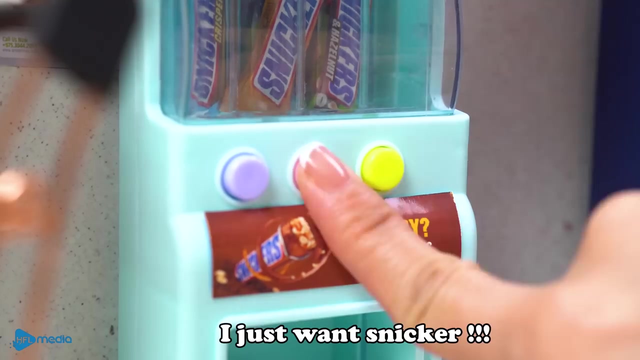 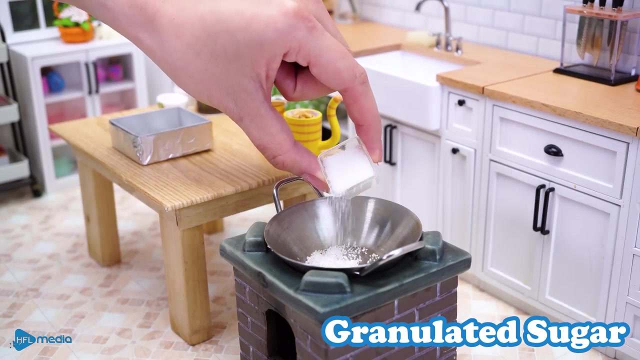 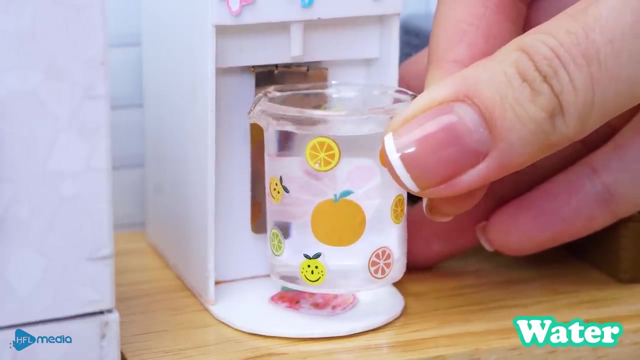 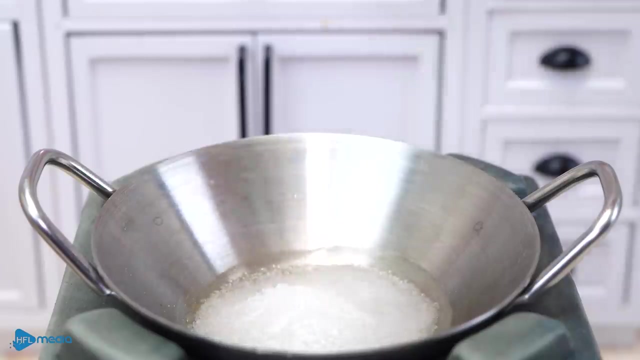 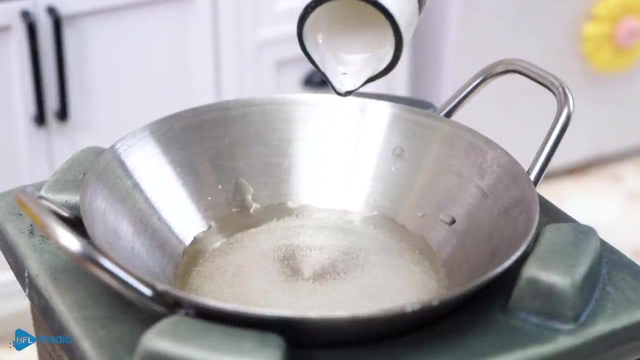 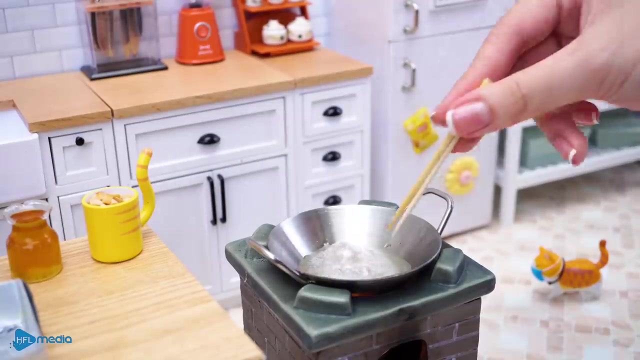 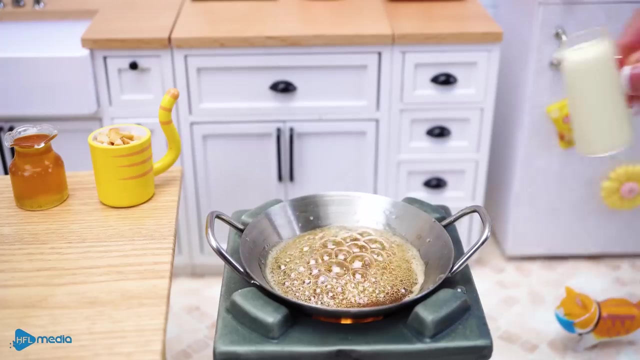 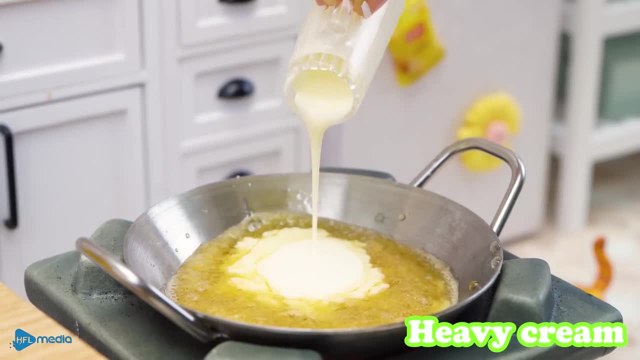 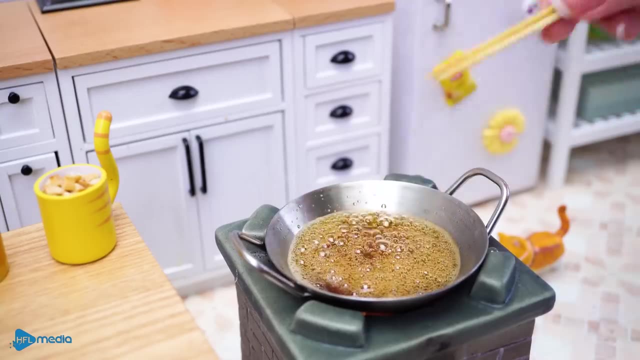 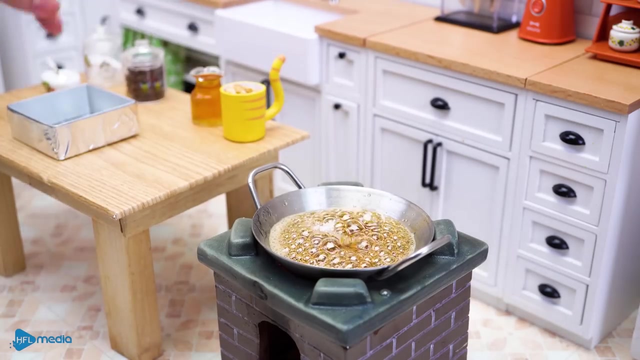 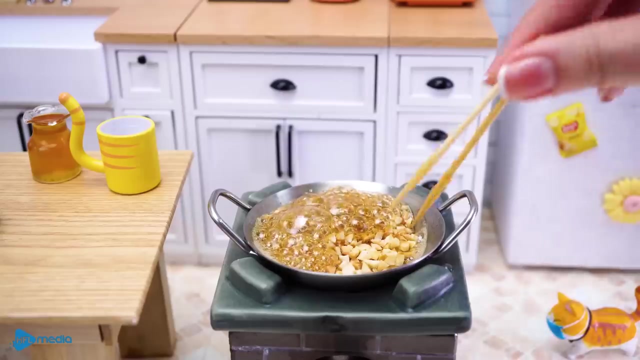 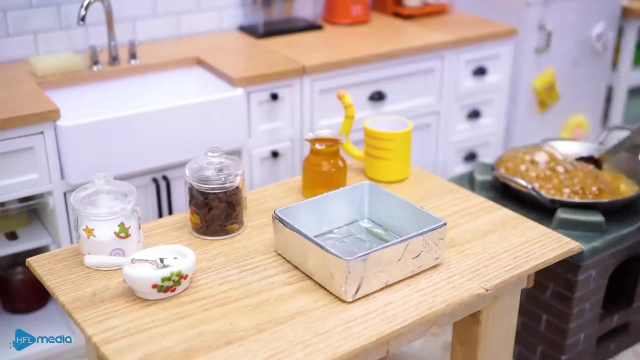 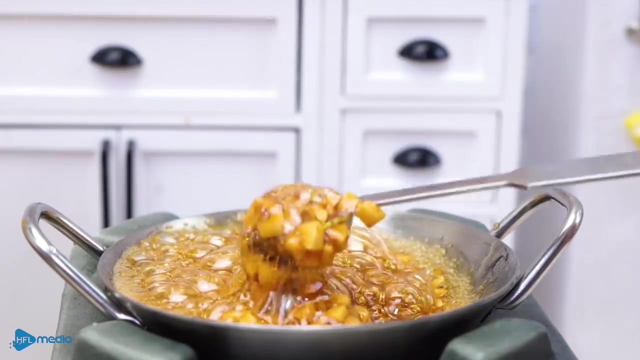 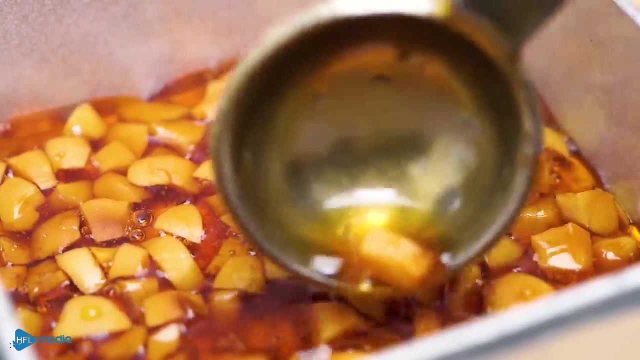 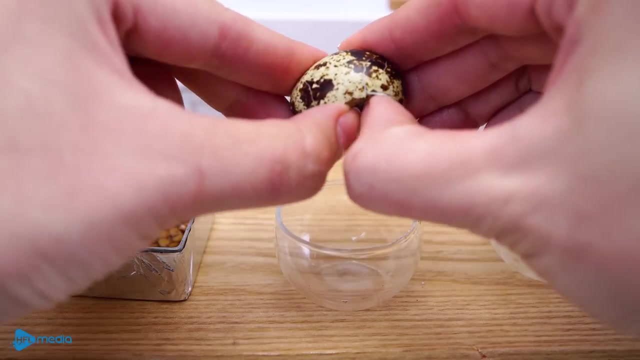 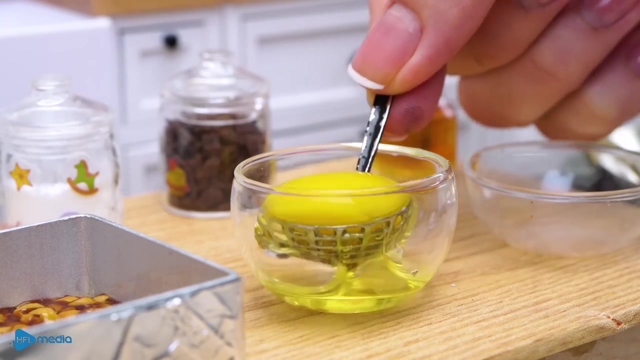 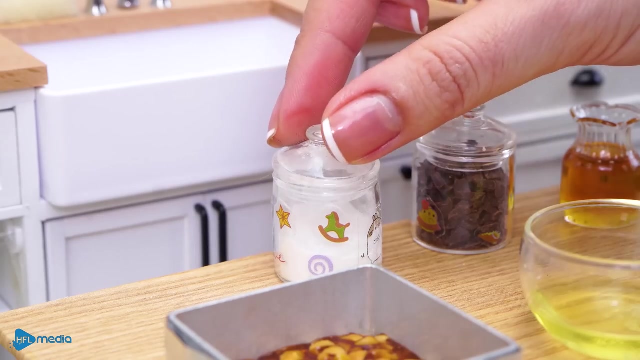 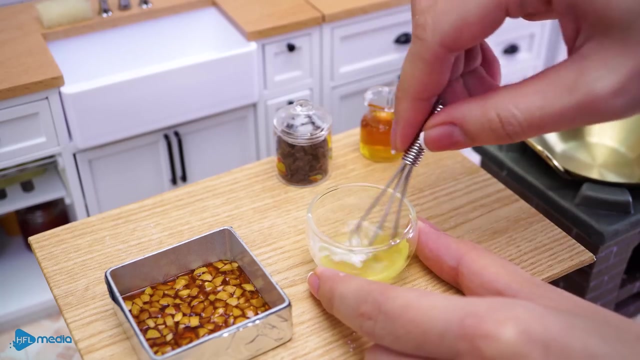 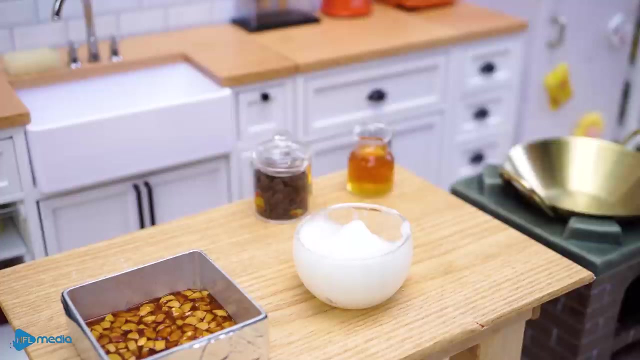 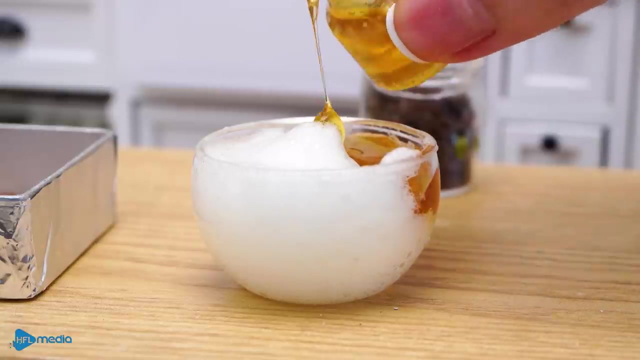 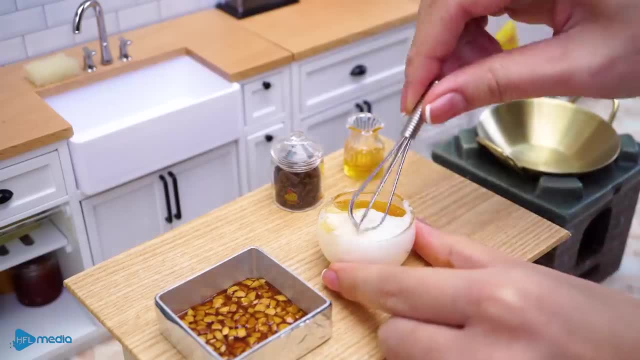 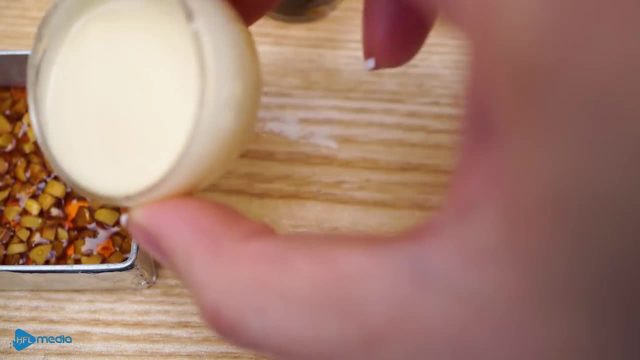 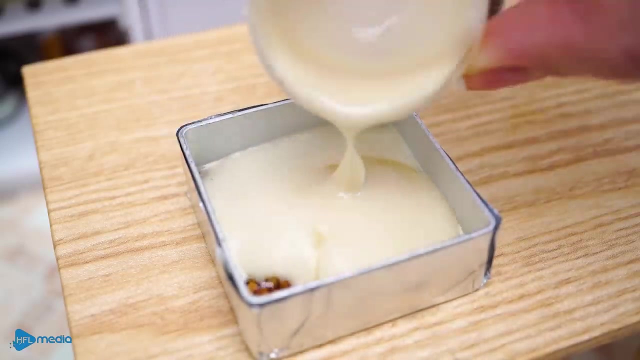 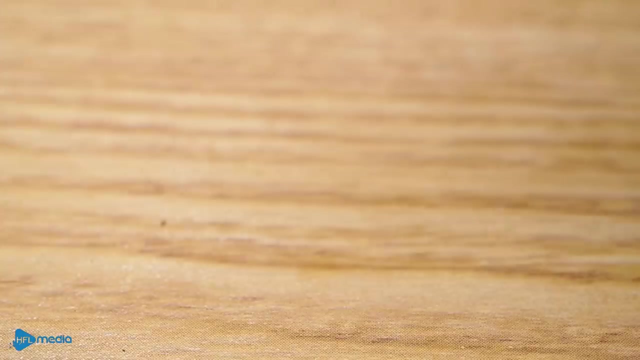 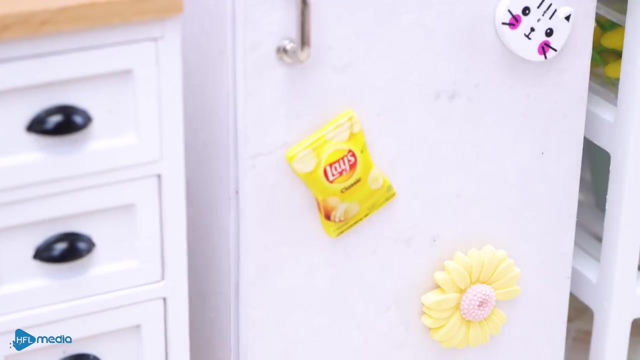 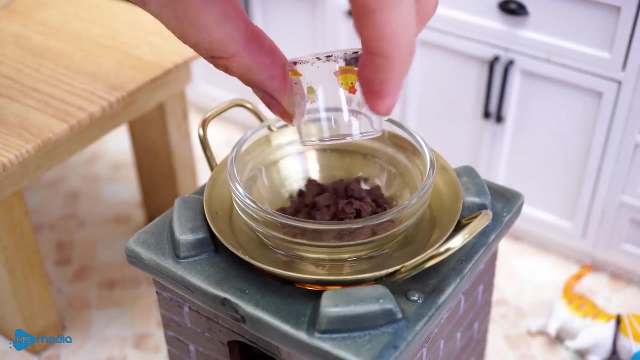 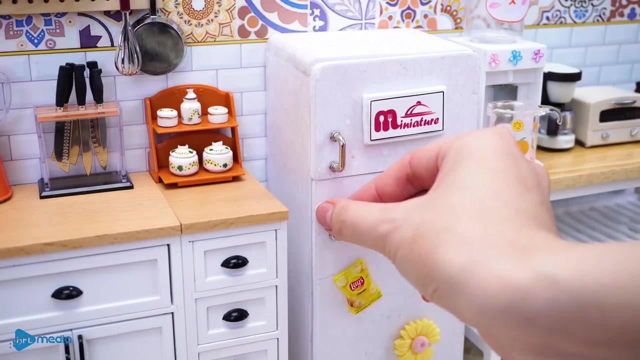 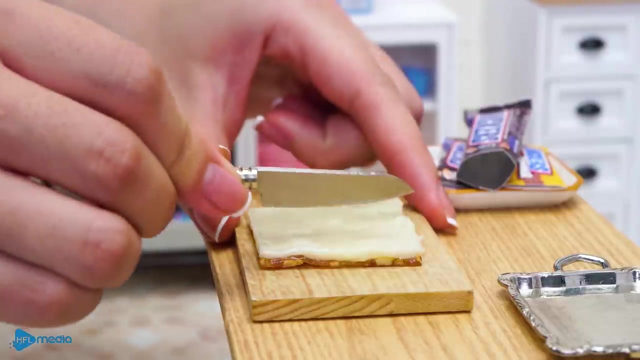 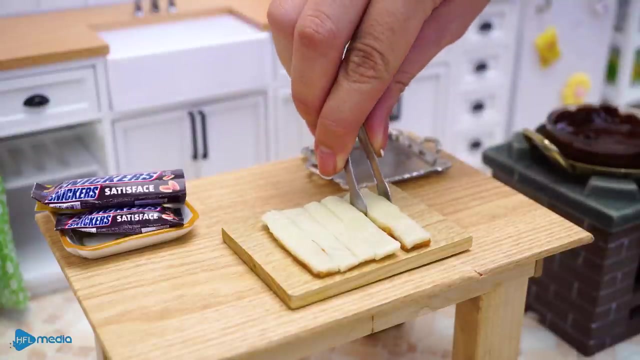 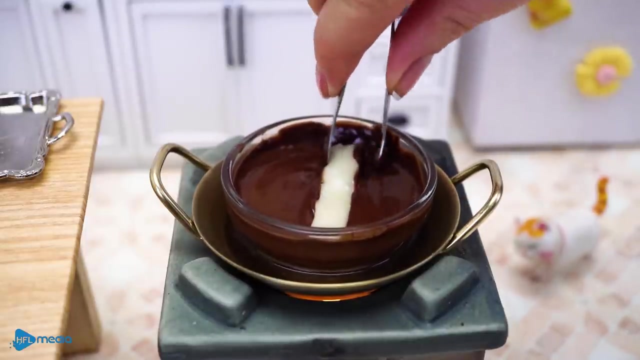 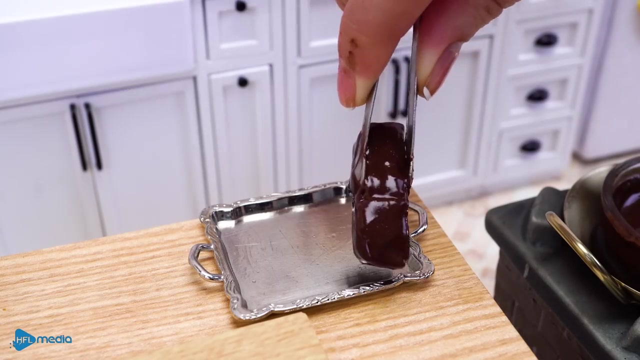 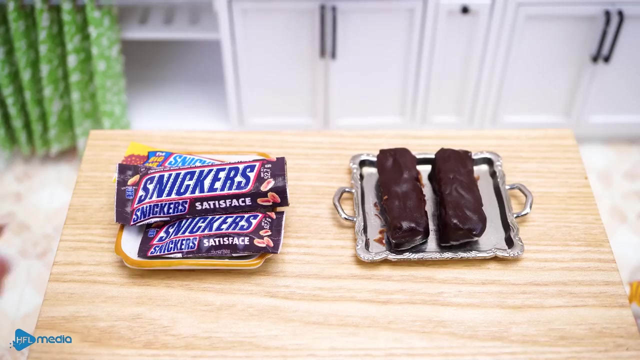 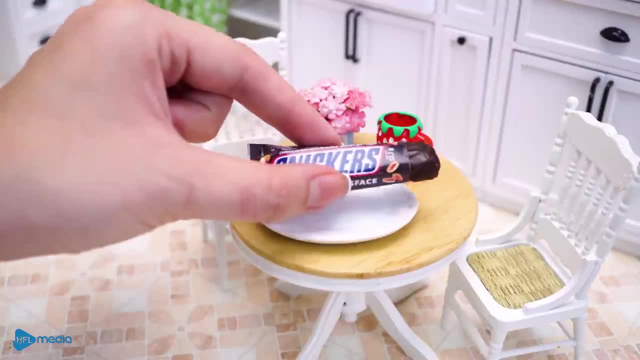 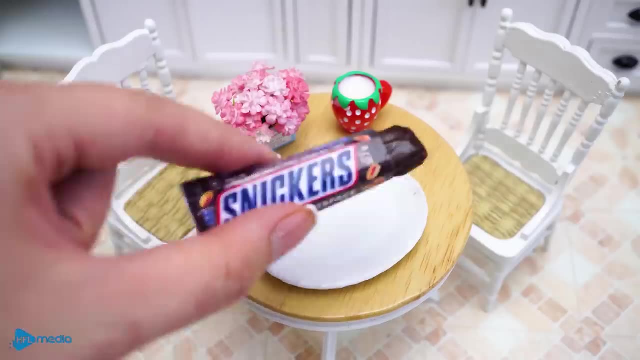 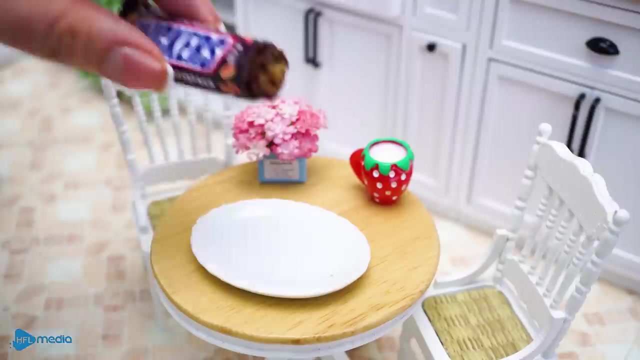 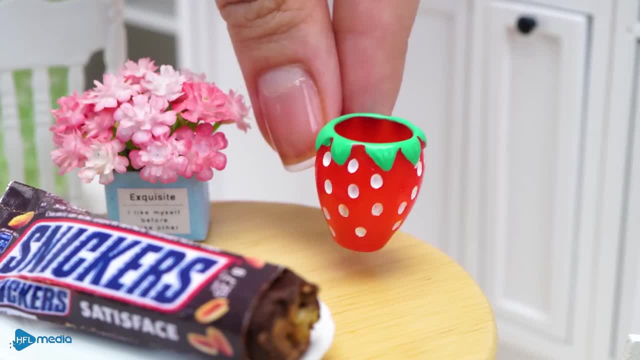 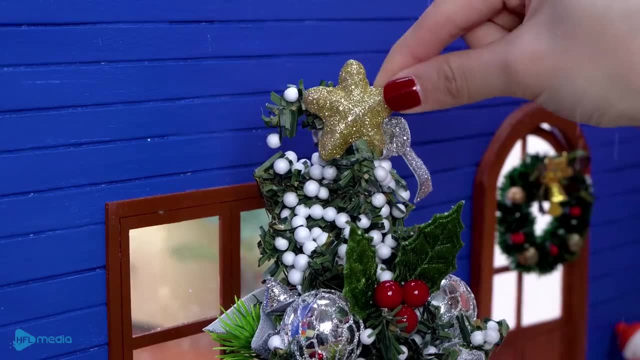 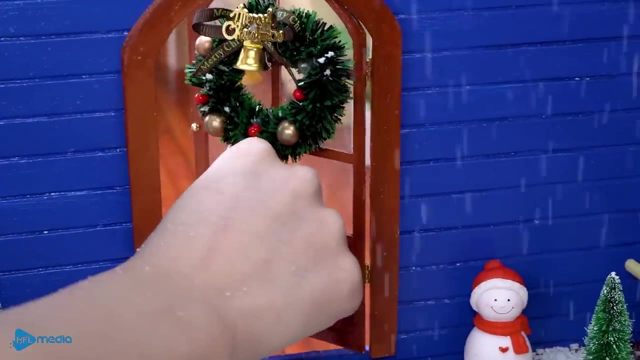 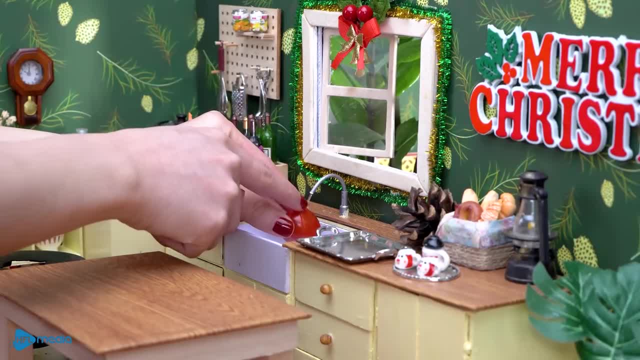 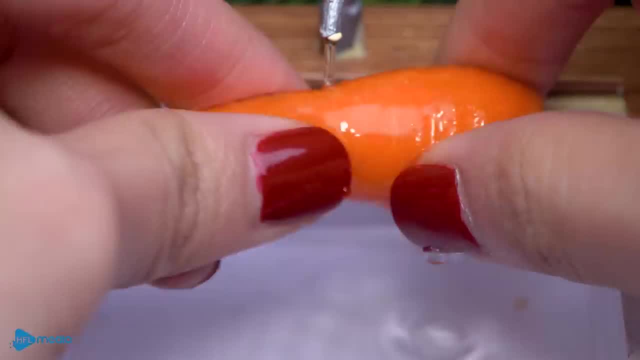 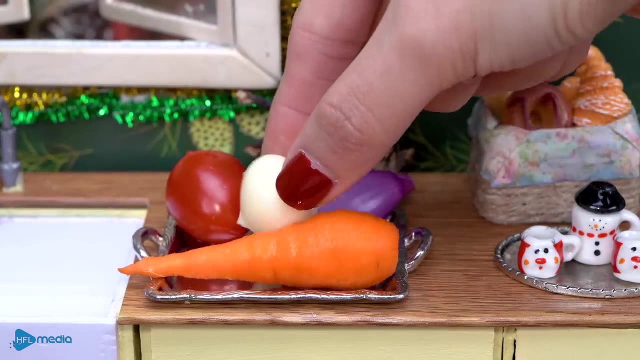 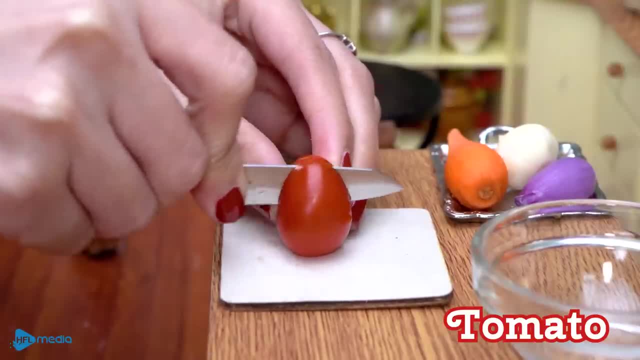 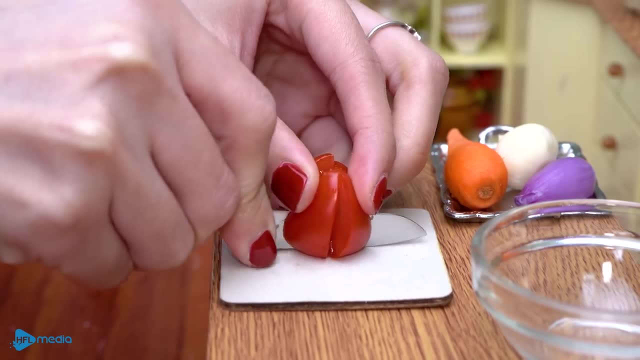 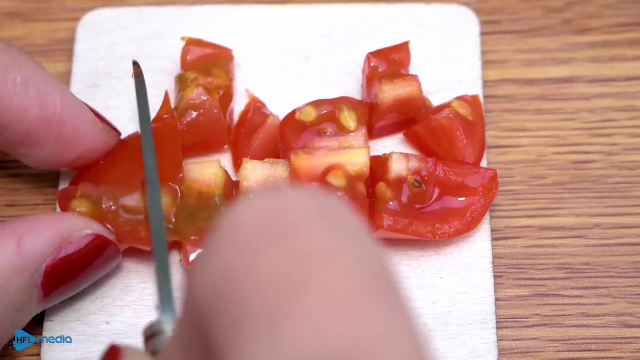 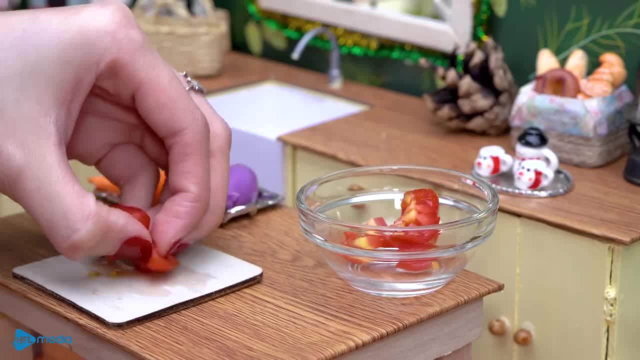 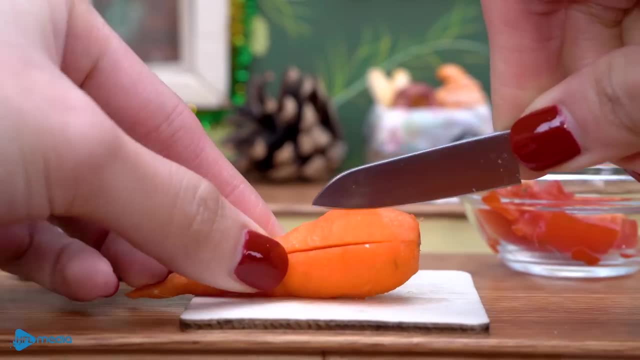 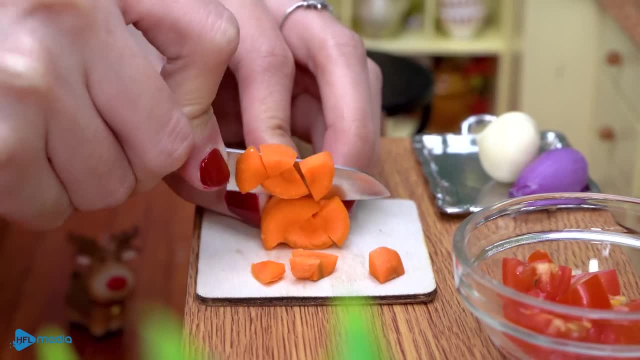 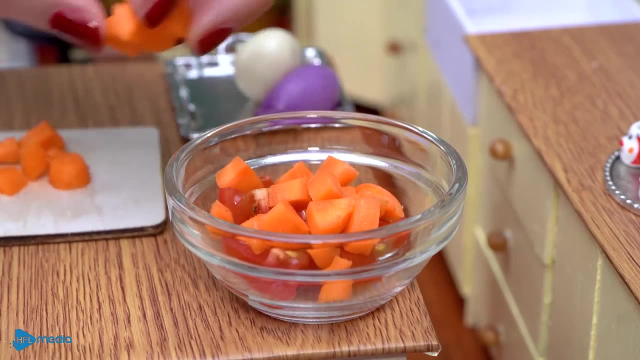 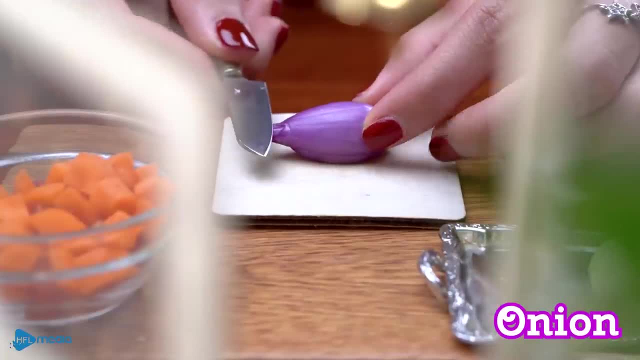 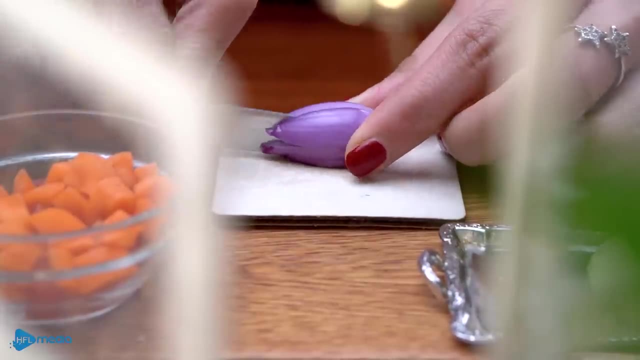 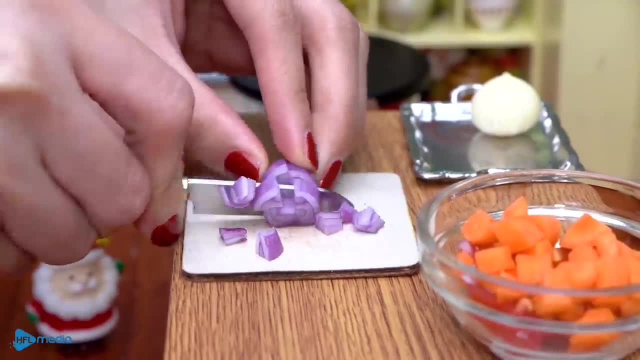 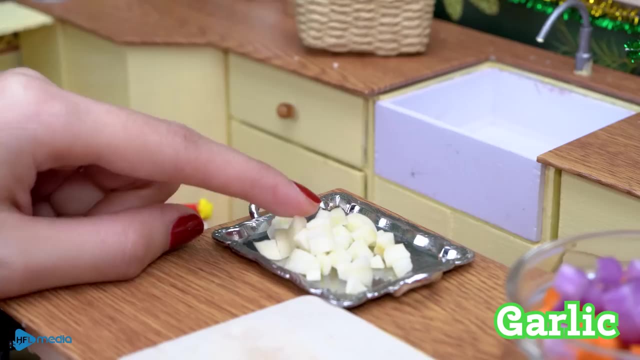 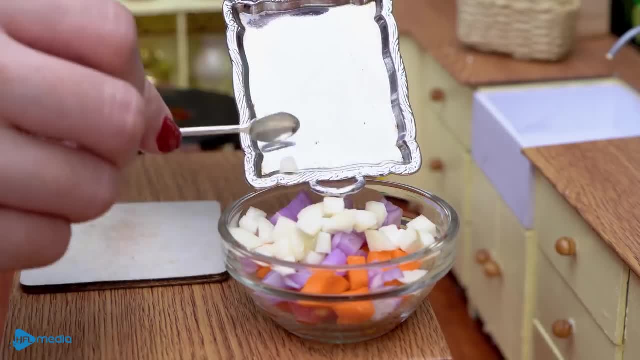 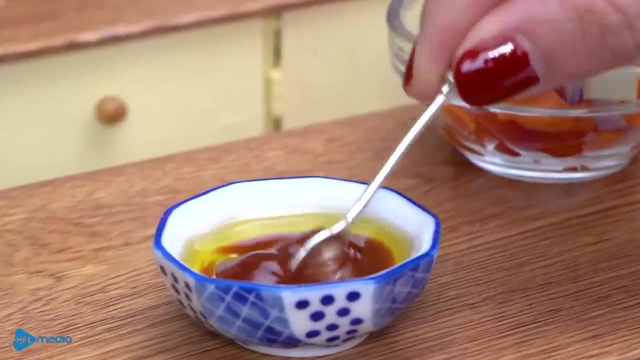 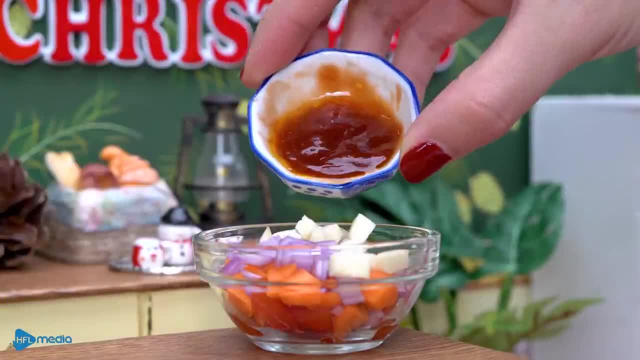 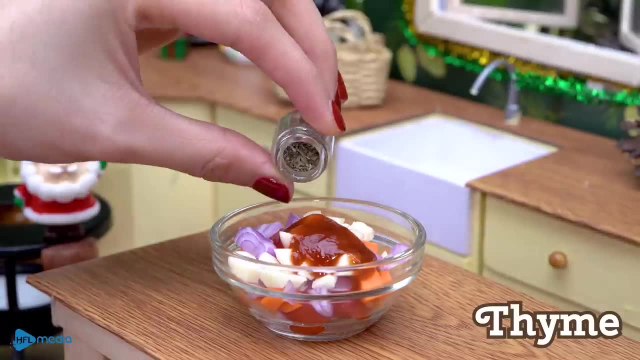 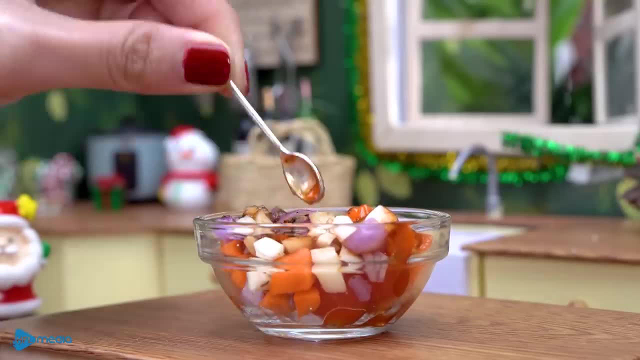 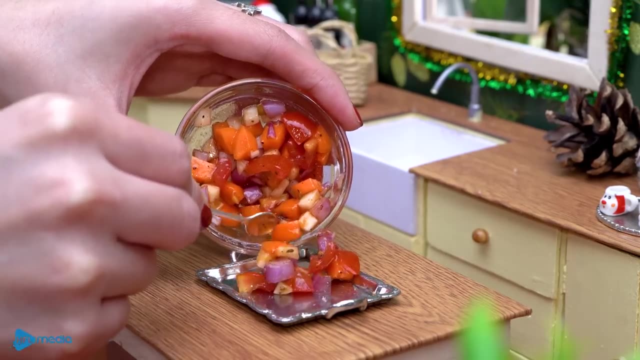 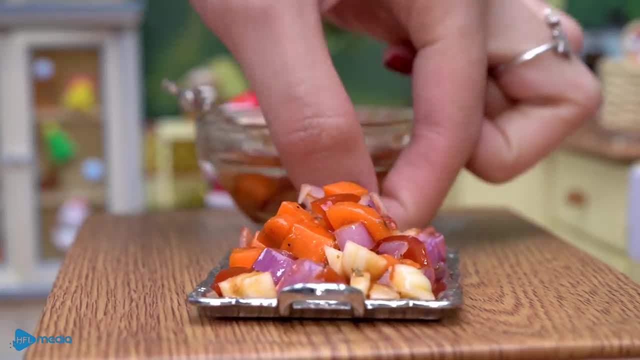 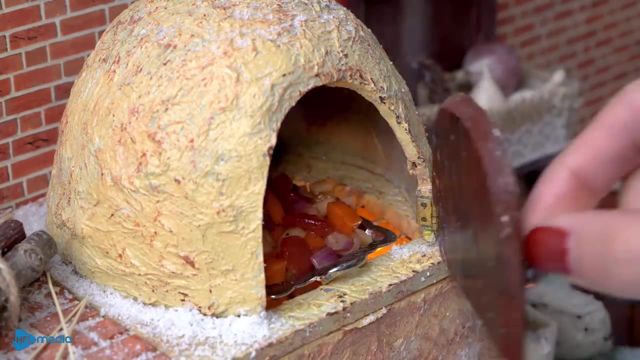 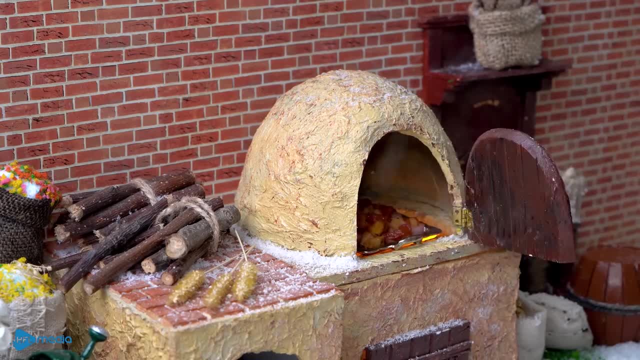 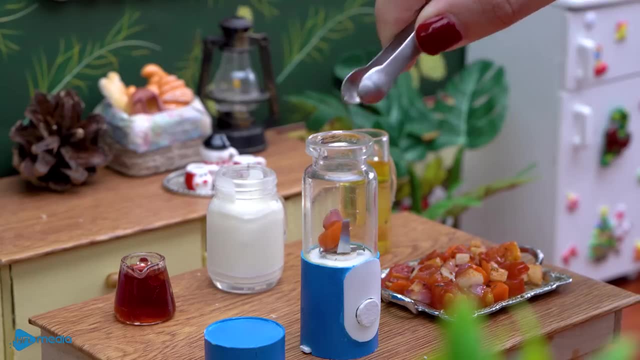 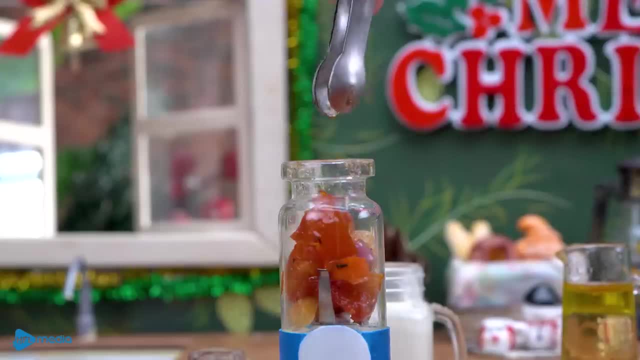 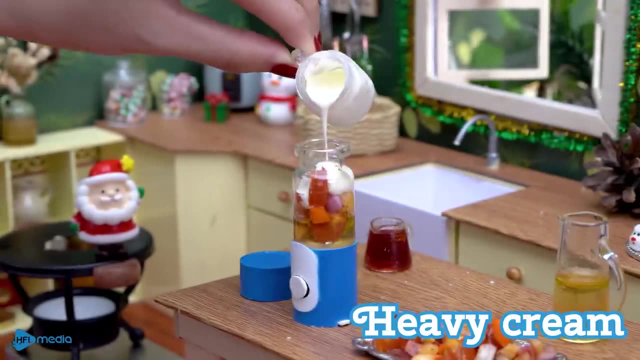 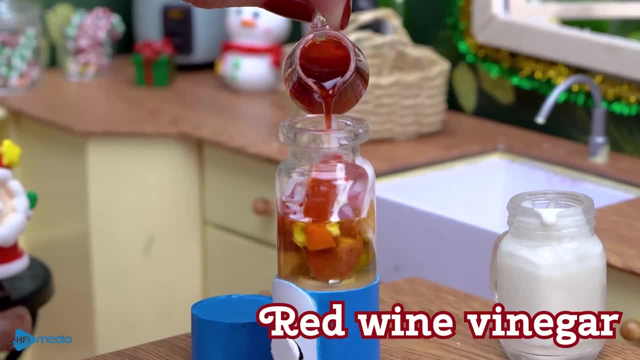 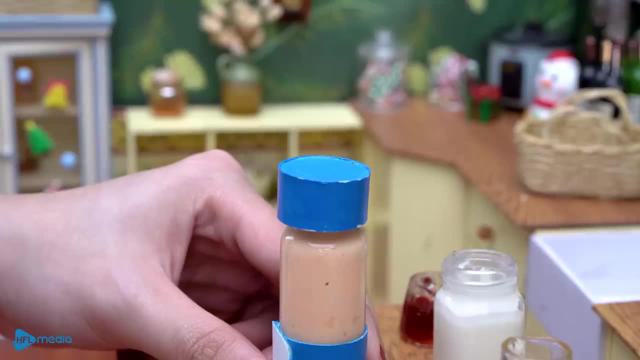 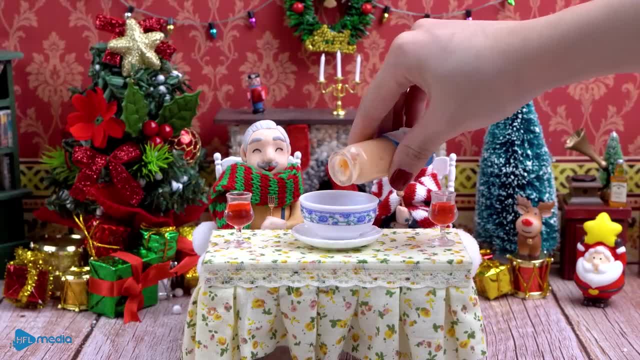 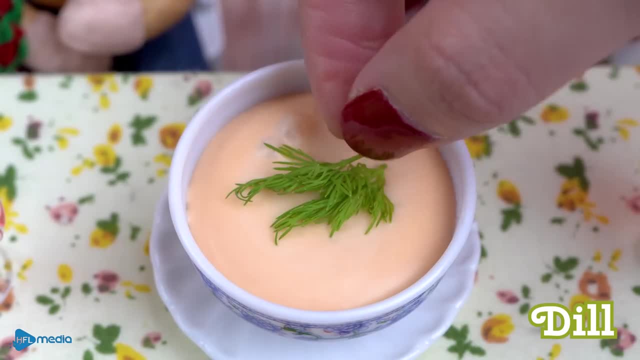 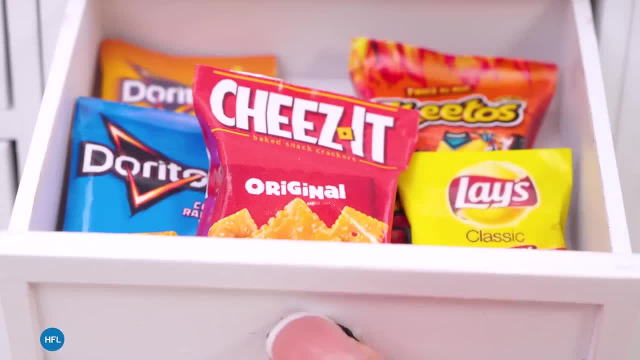 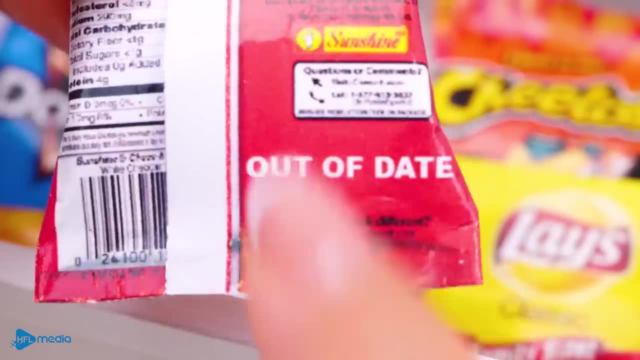 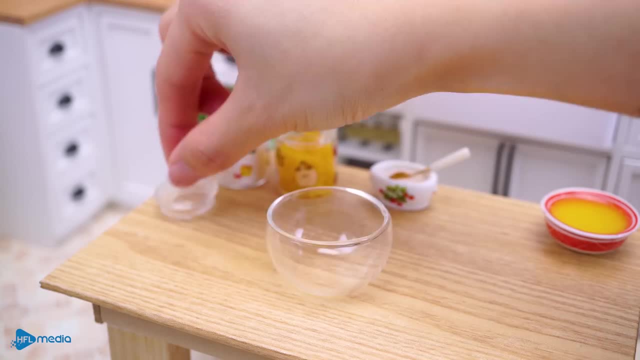 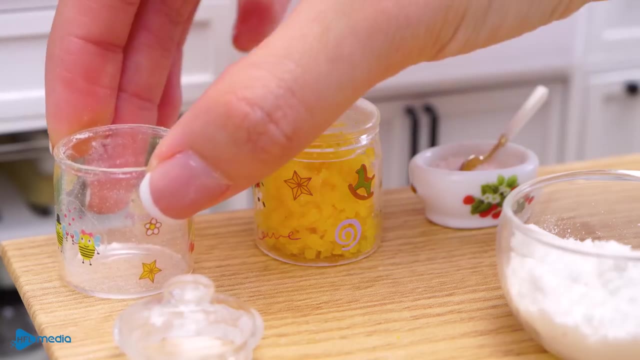 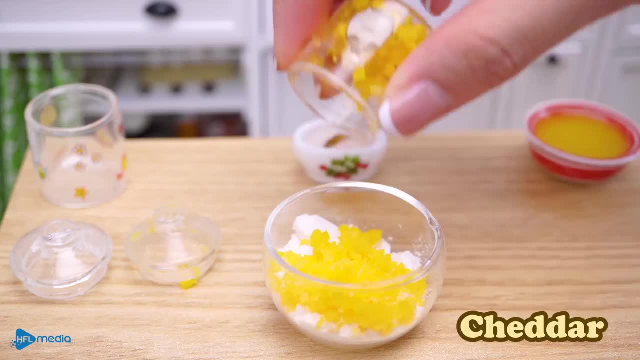 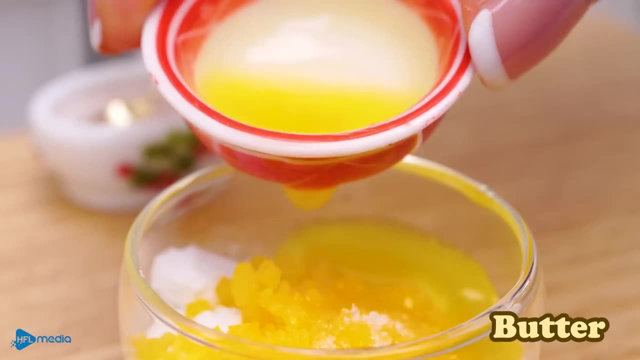 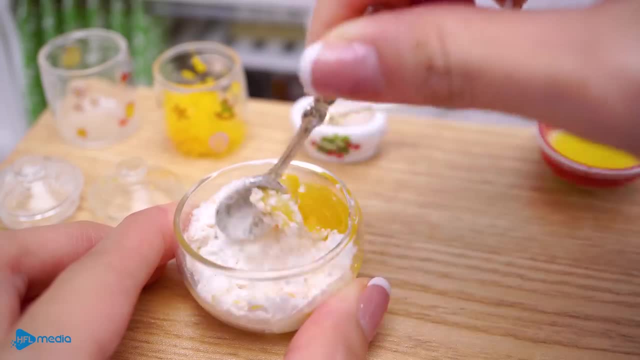 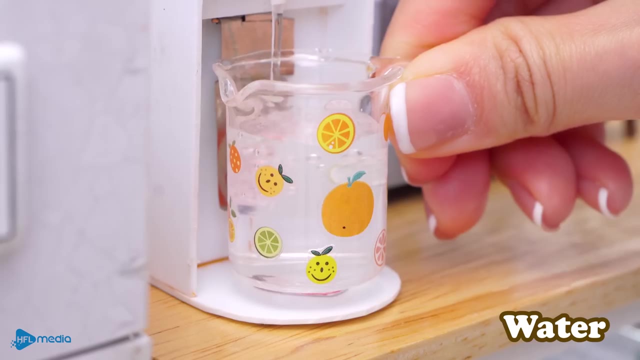 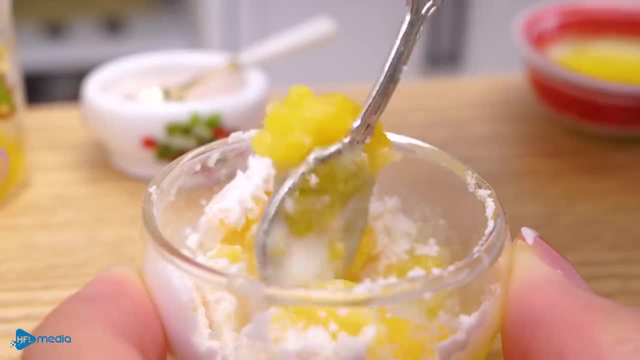 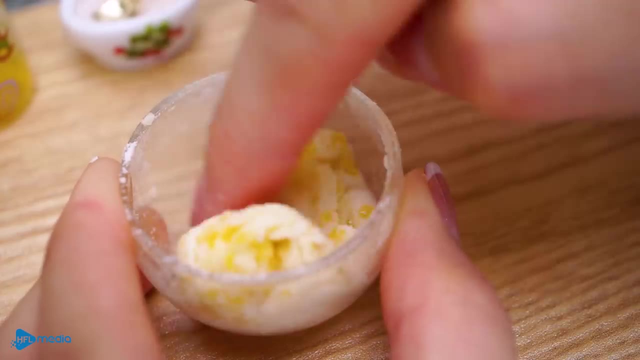 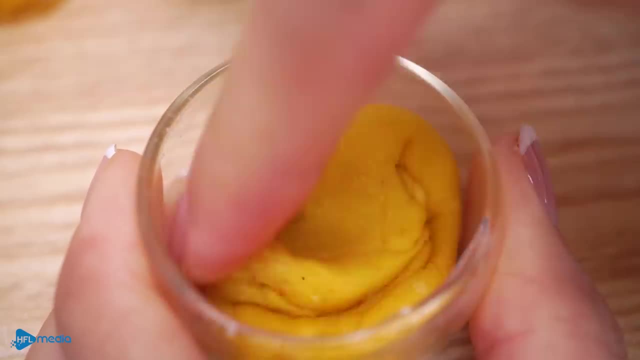 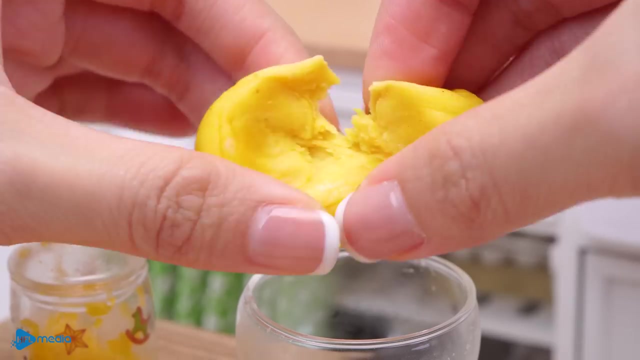 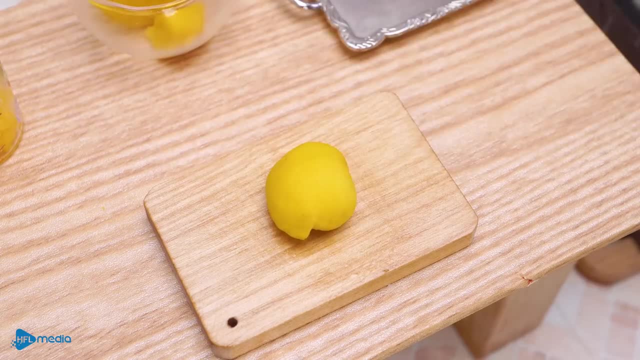 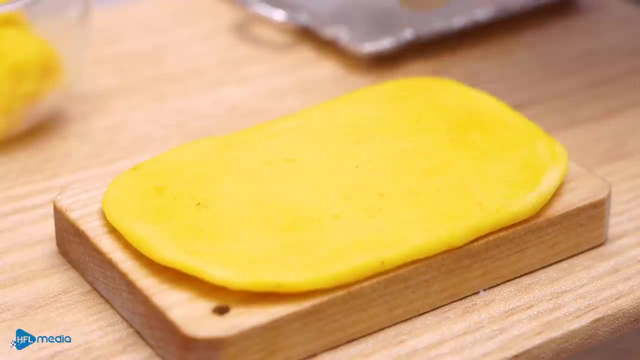 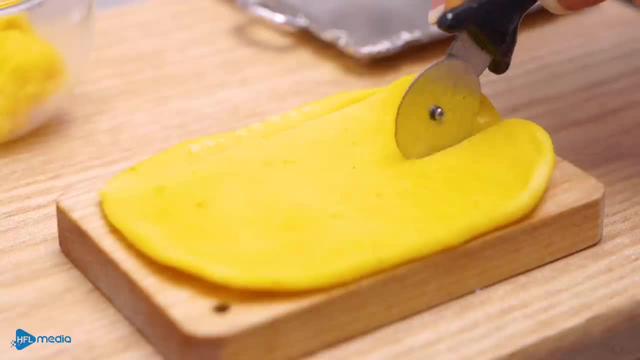 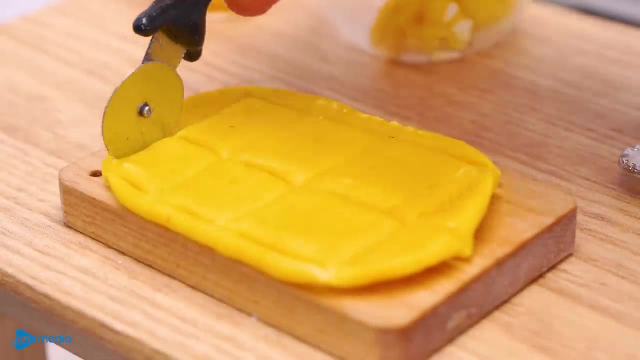 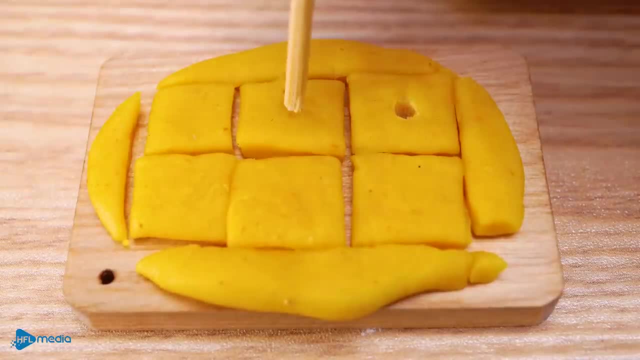 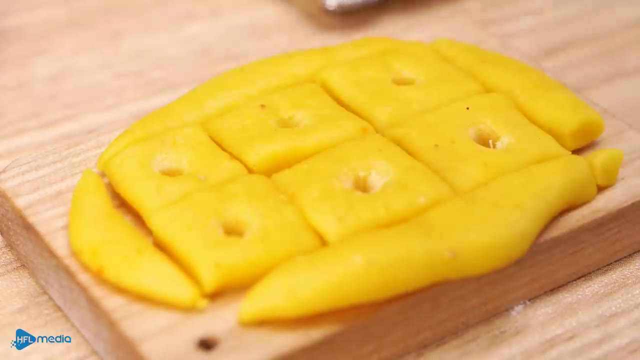 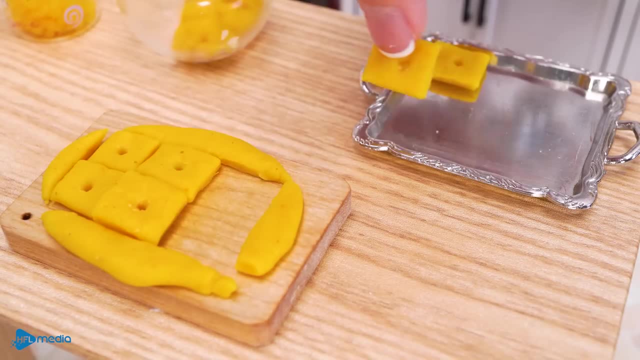 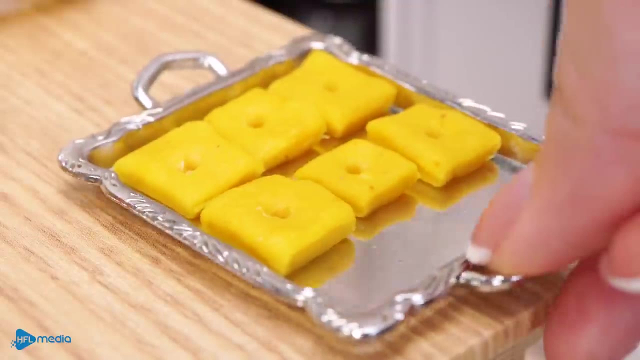 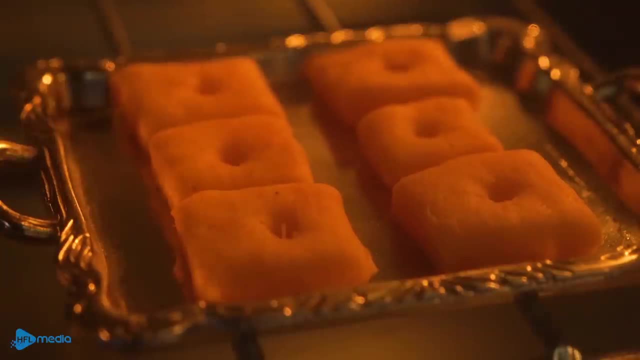 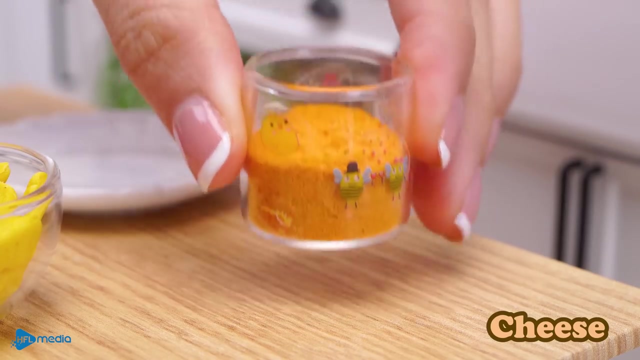 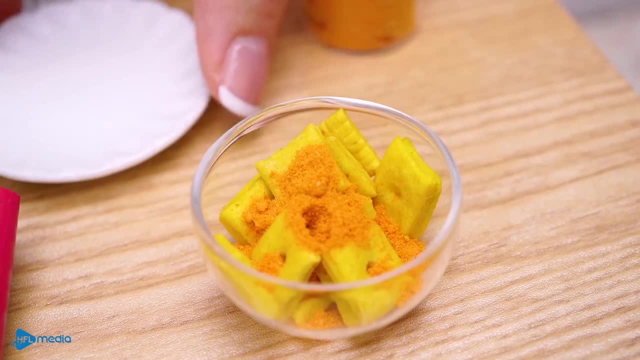 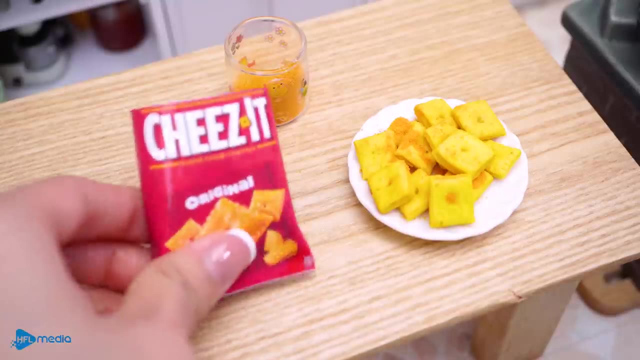 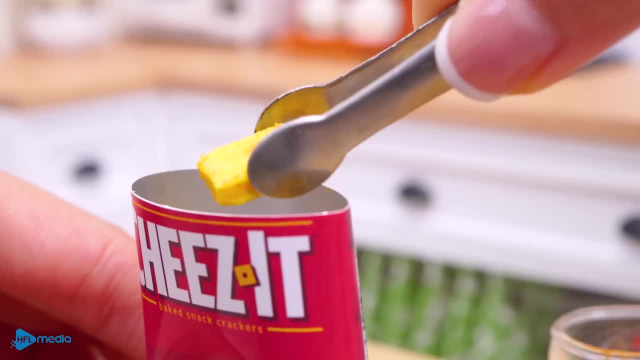 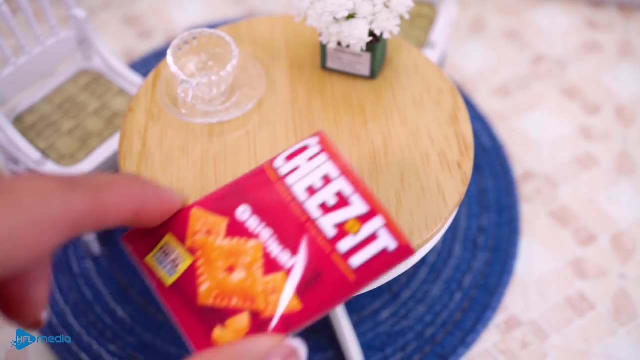 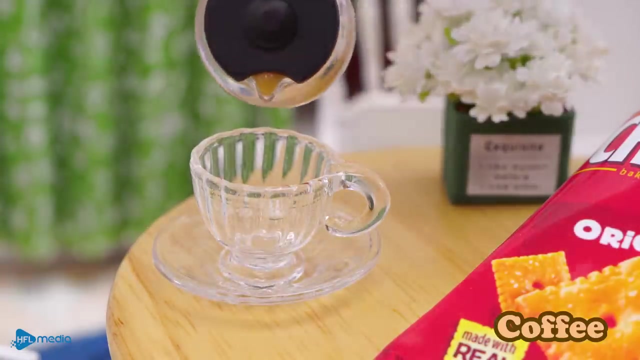 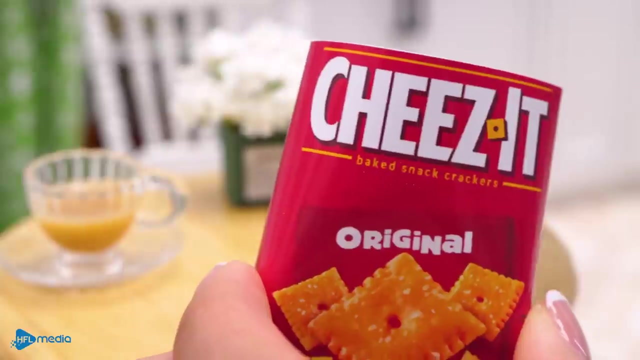 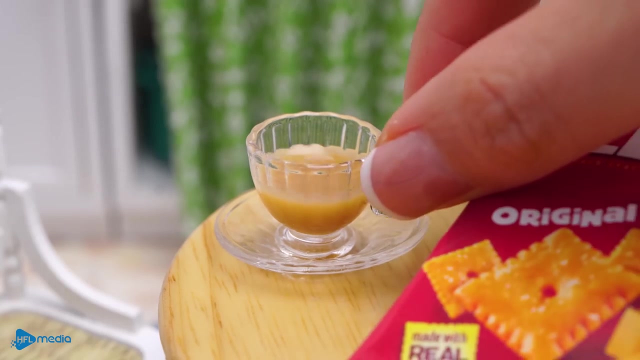 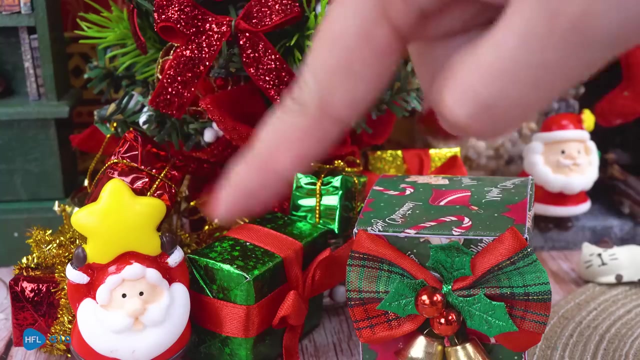 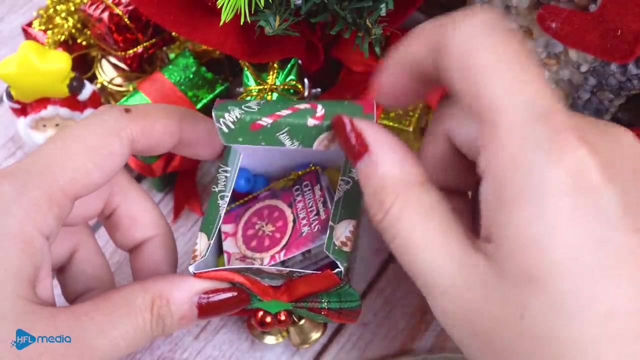 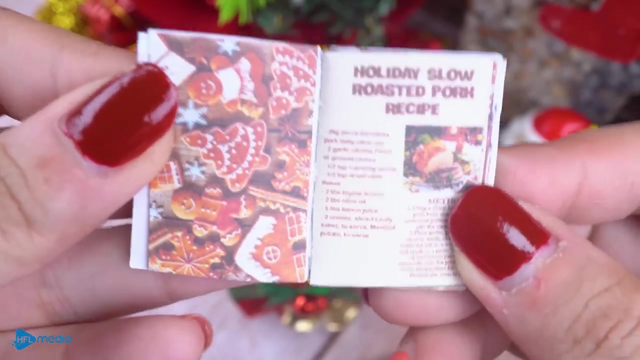 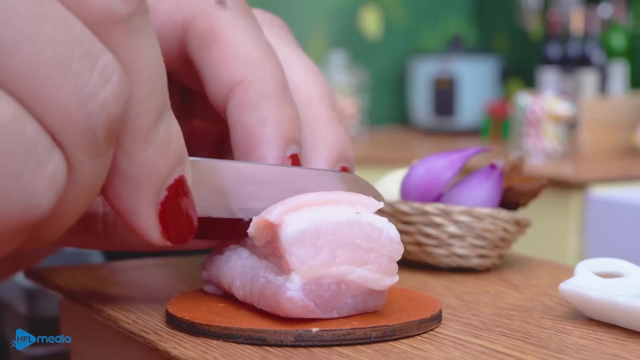 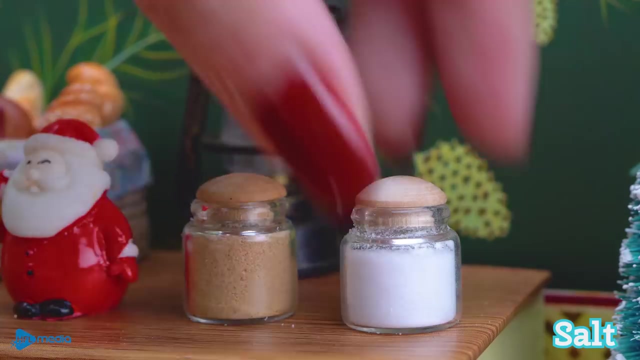 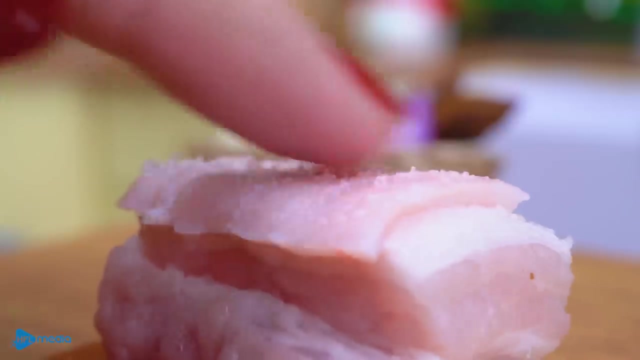 It's rollable, I eat it with ignoreers And I'll finish it today. Come on, I like it. Okay, I choose this one. Wow, I love this present. Let's get started. Okay, I choose this one. 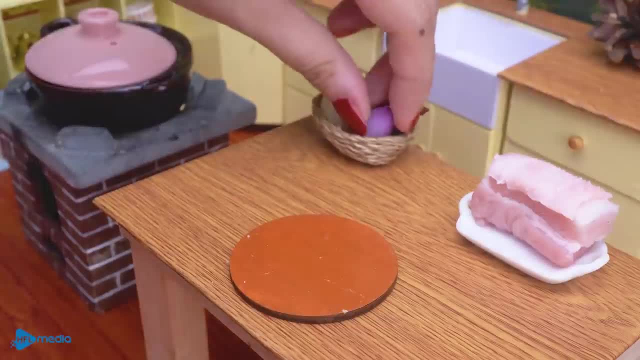 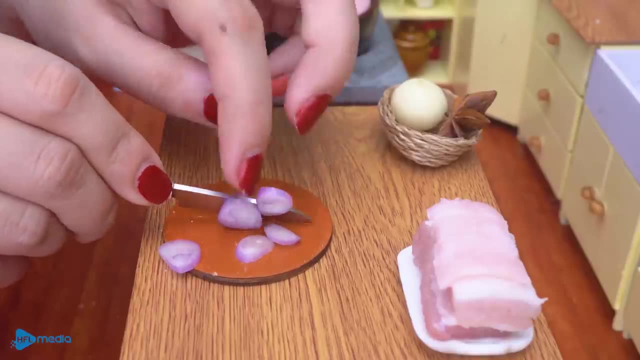 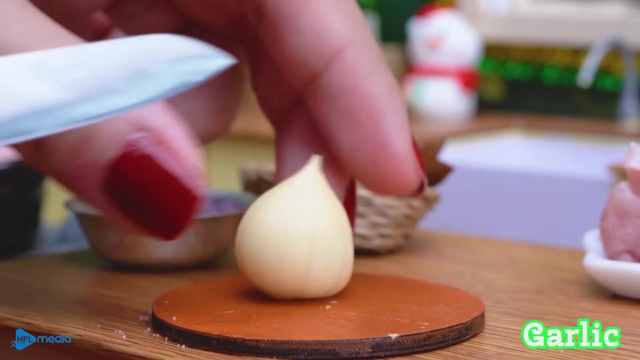 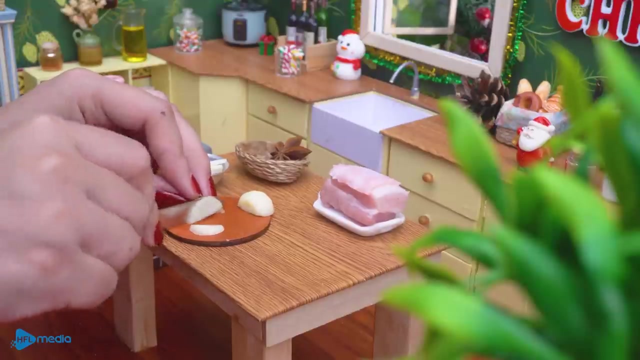 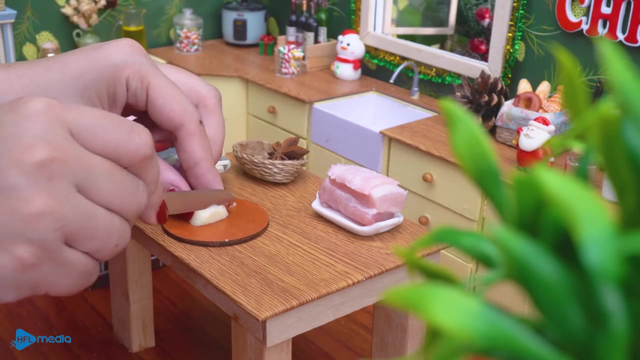 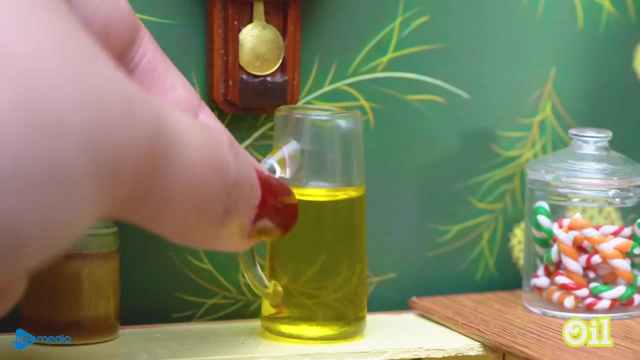 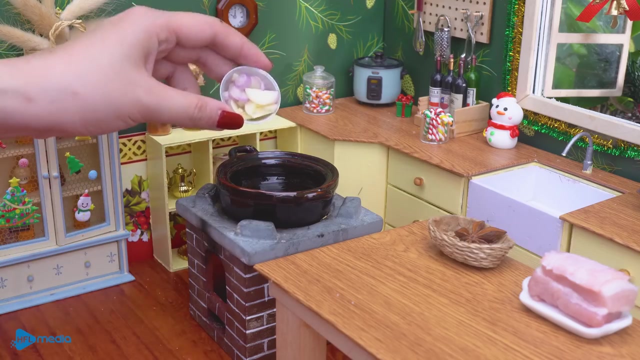 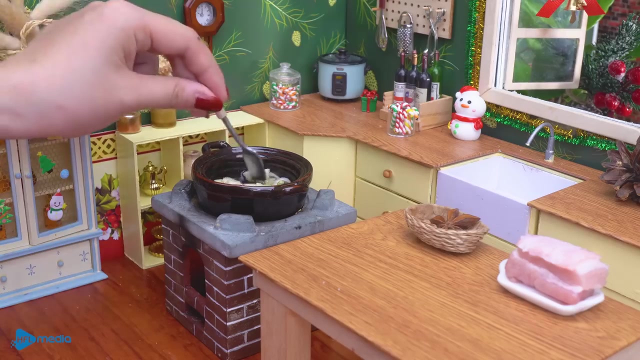 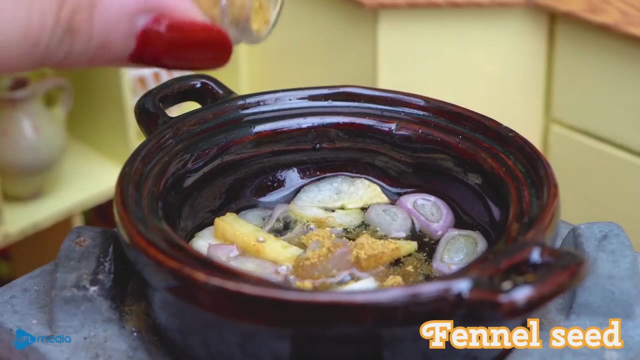 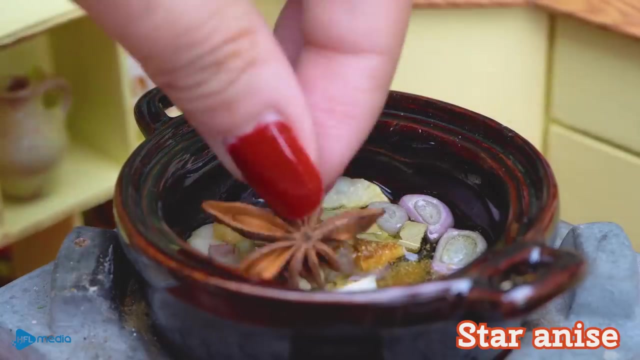 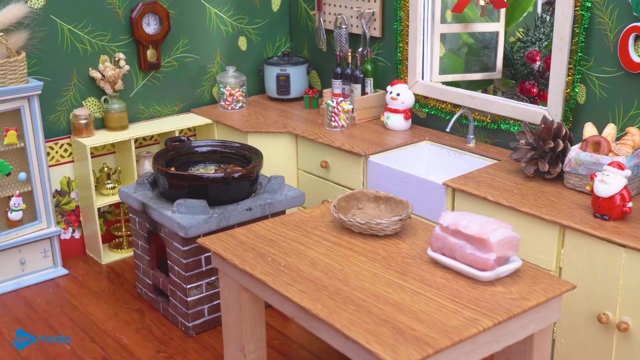 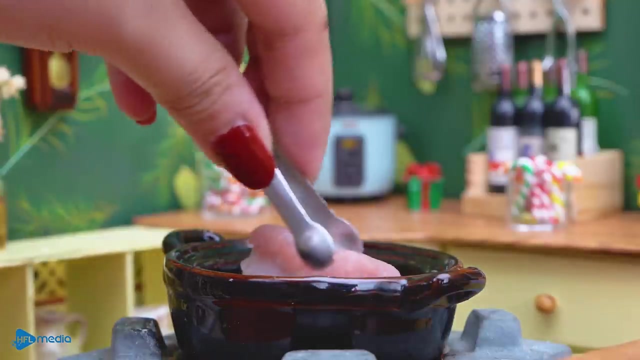 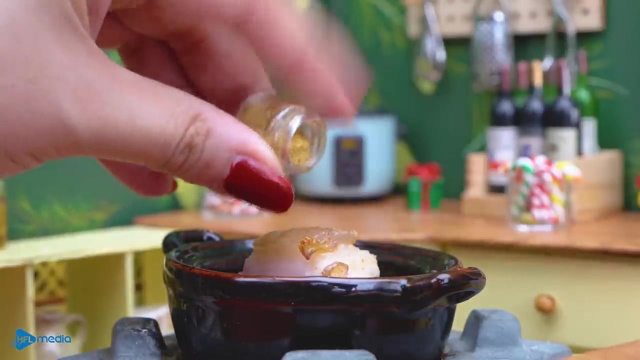